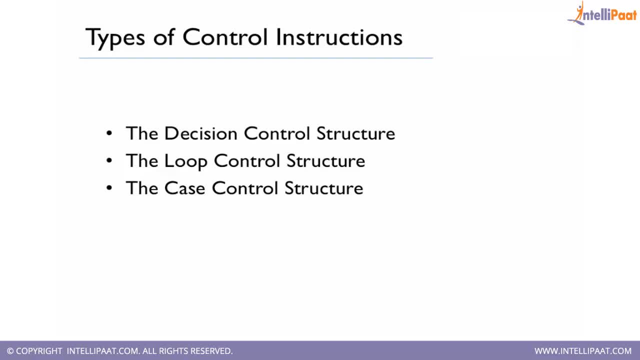 So these are two different actions, whether I will be getting candies or I will not be getting candies. So these kind of statements or these kind of flows comes under decision control structure, Loop control structure. Loop control structure basically comes under events where we require actions more and more. 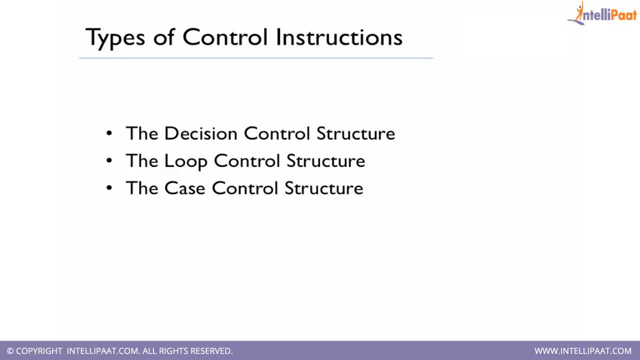 than one time. For example, I want to print table of 10.. So what I have to do? I have to do calculations like 10 into 1,, 10 into 2, 10 into 3.. I need to do it 10 times. 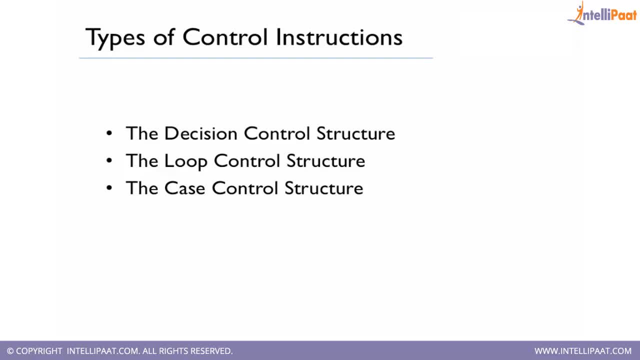 So there are two approaches. One basic approach is like I will write those 10 statements And print my output. So what is the disadvantage of this? because every time, if I want to change the number of times- suppose I want to print 10 into 20, then again I need to write all that 10. 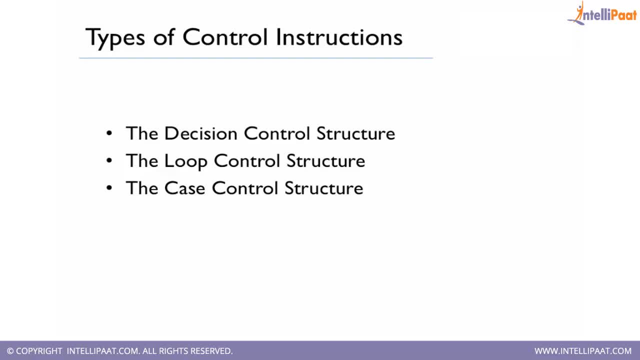 instructions again and again. Instead, if I can use a loop, I just need to loop it around the given number of times. For example, if I have to write table from 1 to 10, I can loop it 10 times. If I want to write table from 1 to 20, I can loop it at 20 times. 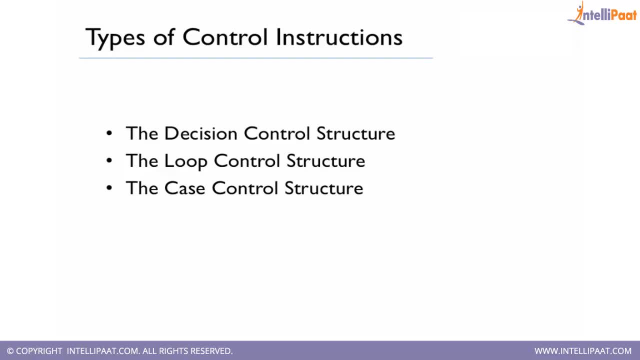 So this gives me more control over my program. So for these kind of things, loop control structures are used. Case control structures are used for decision making. These are the special type of control structures. These are the special type of control structures. These are the special type of decision making structures where the event can have more. 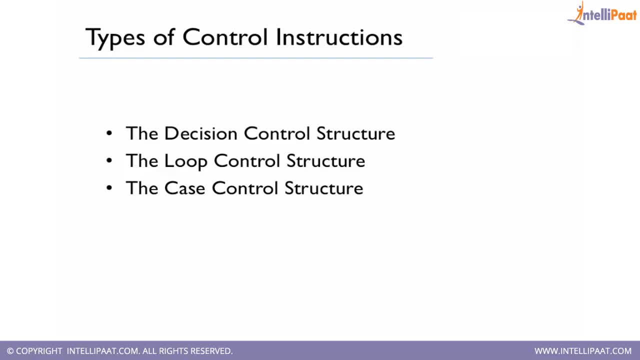 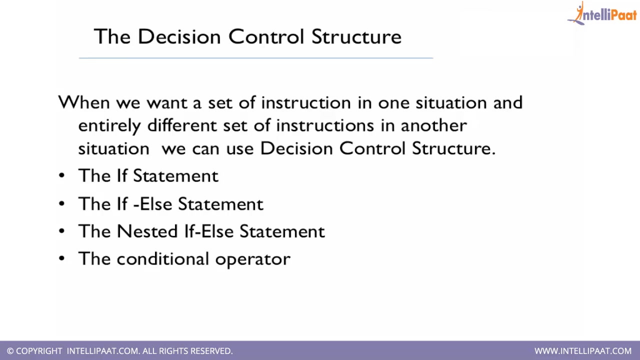 than one output and we need to take action on each and every output. So, using case control structures, we can write a code for these kind of behaviors. So these are the major issues. So here let's see about decision control structure. So, as we have discussed earlier, when we want a set of instructions in one situation and 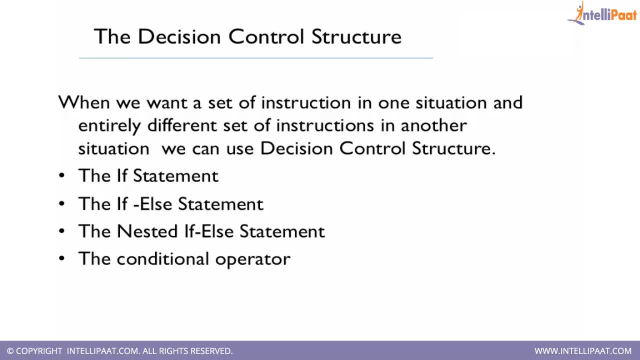 entirely different set of instruction. in other situation we use decision control structure. In decision control structure we have if statement, We have if else statement, we have Nested if-else statement and conditional operator. so what is if a statement? let's see one flowchart of if and else control structure. 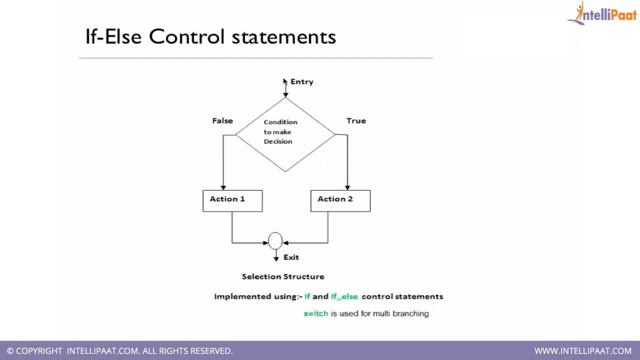 control statement. we will be entering to a program in this manner. this is symbol of decision-making, so condition to make decision. so earlier I have given an example of passing in the mathematics test. so I can say a result of my mathematics test, true means I passed false. 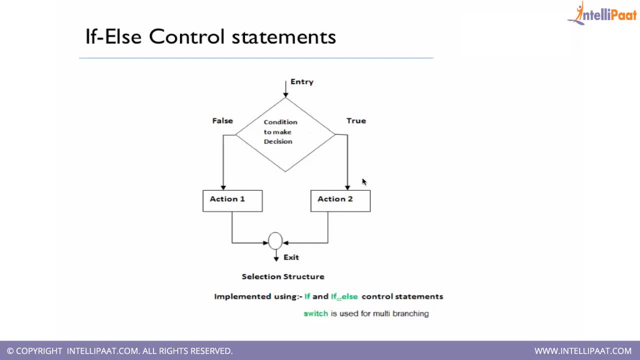 means I failed. so in case of true and we getting candies, in case of false, I will be not getting the candies. so how we can, how we write in our C program, so we write it if condition and then statement or block of statements. so in this it can be either one statement or many. 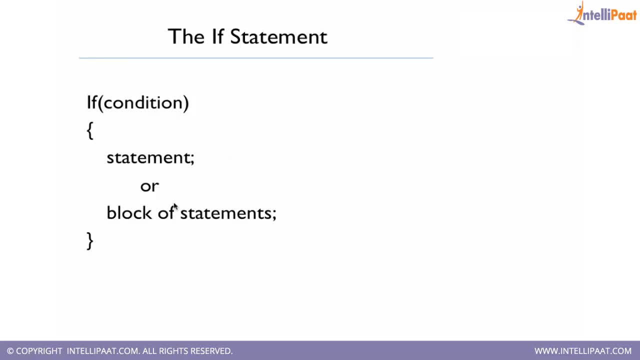 statements. that's why we have written block of statements. okay. so let's try it out. let's do some dry run of this code. let's predict what should be the output of this program. okay, so I am declaring a variable a equal to zero. I will be entering a number. okay, user will be giving. 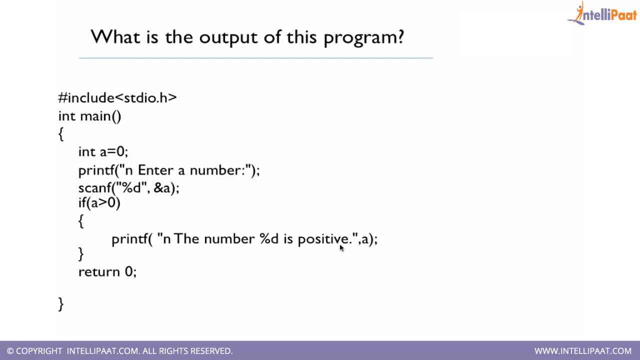 me a number. if a is greater than zero, I'll be printing. a is a positive number and it turns you. so what this program is doing? it accepts one number from the user and check if the number is positive or not. okay, so let's write a code for this. 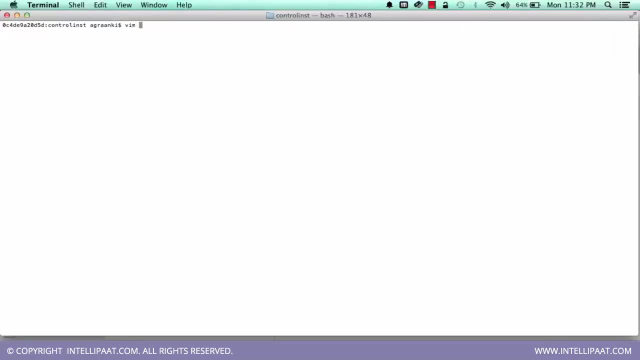 ok, let's create file. okay, to check if number is greater than zero, then zero or zero number is positive. let's include stdioh hash include. let's write the main method so we return zero. okay, now let's declare one integer, a let's printf and: 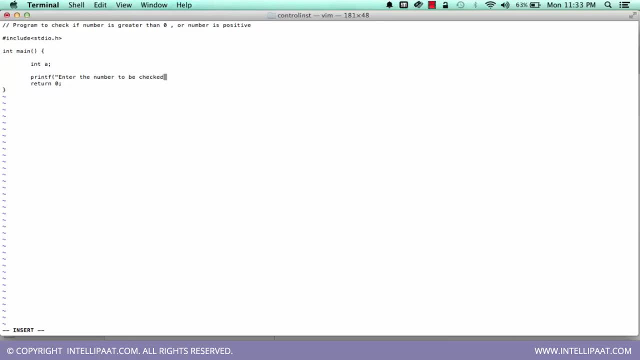 number to be checked: canf, %d, %a. so we'll be getting a in this. okay, here I missed double quotes. okay, now I'm writing: if a is greater than zero, then print: this is statement: yes, the given number is zero, okay, else, number is not greater than zero. okay, let's do one printer so that we differentiate between our output and 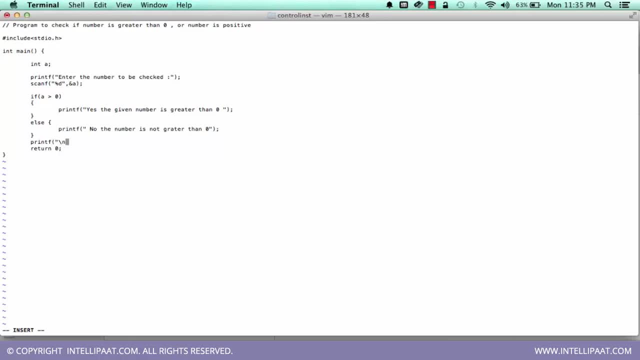 our thanks, slash n? ok, let's save it, just compile it ok. compilation is success, let's run it. ok. enter the number to be checked. I enter three, 504, com最後三. enter the number to be checked. I enter three, 504, comlessor number to be checked. enter three, 504, 1.ん. 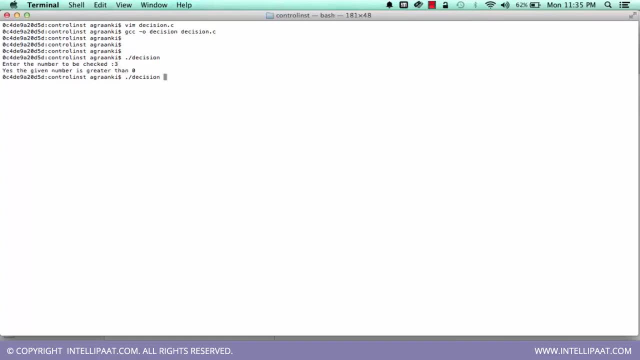 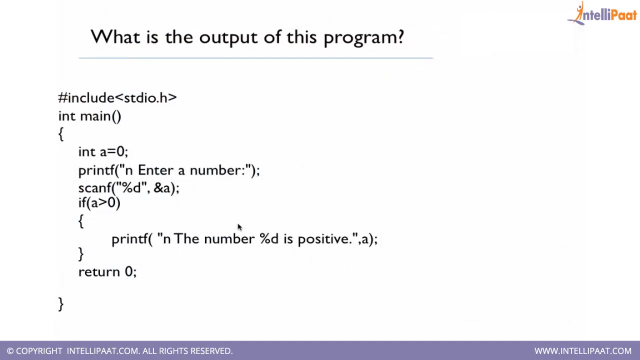 it says: yes, the given number is greater than 0. let me run it again. I'll give minus 4. say: no, the given number is not greater than 0. so this is how we use if statement. here I have used if and else, so both are related, like if you don't. 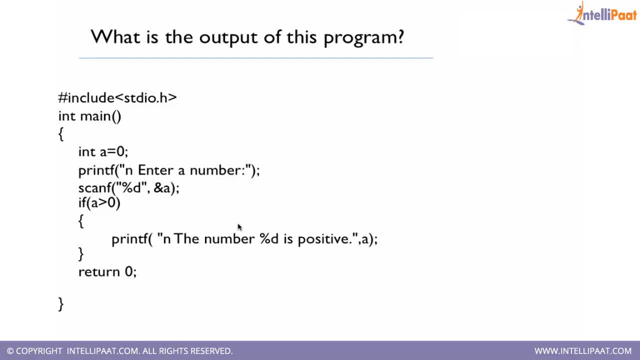 use else statement, then it is considered that you don't want to do anything if the condition is false, so what? it is better if you write else statement so that in case, if your logic does not want you to do anything in else statement, let's keep it empty. it would be more clearer. 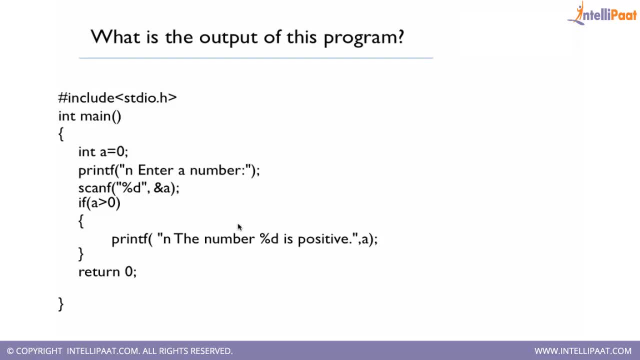 and future. if you want to use it, you can write some code on this or you can have some printf in the else's statement saying that the condition was false. so we, so else's statement is printed. so this will be helpful while doing the debugging, if any, if you, if anything is not correct and you are debugging even. 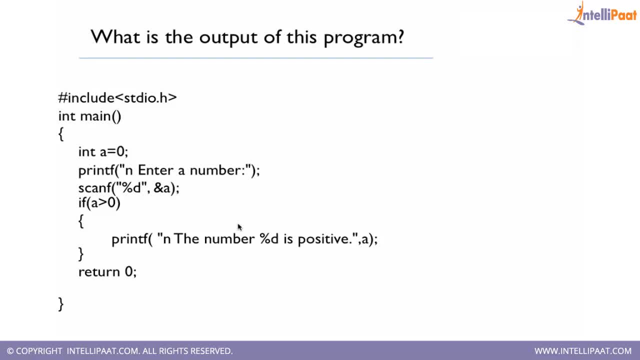 check the logs and see, okay, why your program is misbehaving. so it's good to have else condition, okay. so this is the if and else condition that we have covered in the example. so if condition statement 1, else condition statement 2. so in the code that we have written we have checked: if a is greater than 0, then 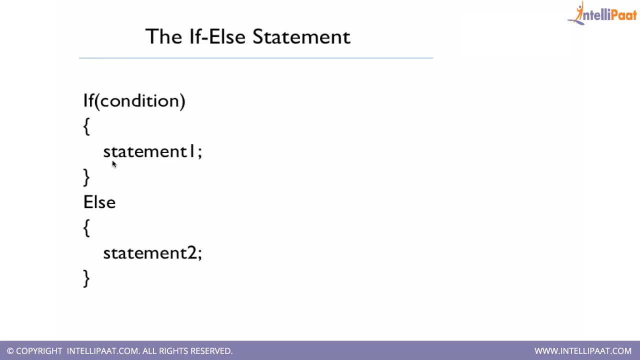 statement 1 is executed. the statement 1 was: printf- yes, the number is greater than 0, else printf no, the number is not greater than 0. okay, so here is one more example. write a program to determine if a given number is even or odd. so this program is much. 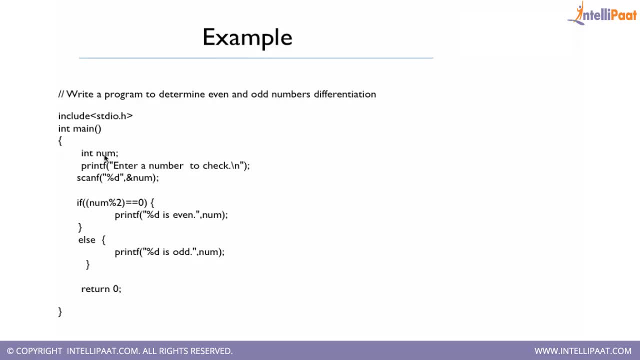 more similar to what we have already written, will be having a number, will be any, will be declaring an integer variable and getting it from the user and checking if, if, checking if the modulus or modular operation of the number by 2 is giving 0, if yes, then we say that number is even else. we'll say 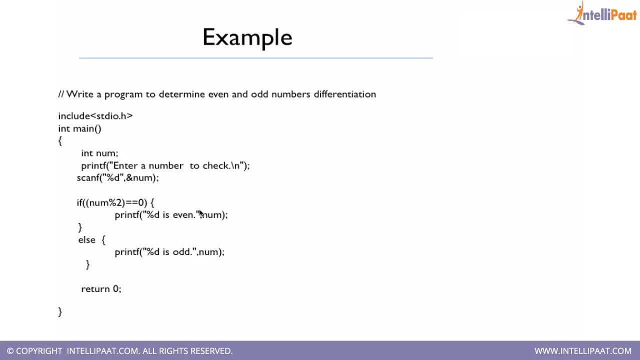 the number is odd. so when there is a complete code, I like you if you just try it out by yourself and get more familiar with if and else statement. so nested if else statement. nested if else statement has one extra thing which is called else. if so, if condition 1 is true, then statement 1 is executed. if condition 1: 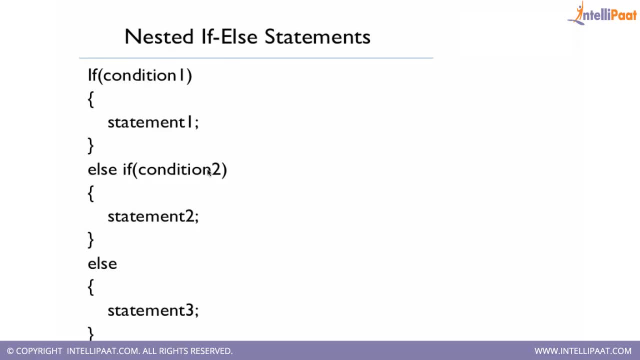 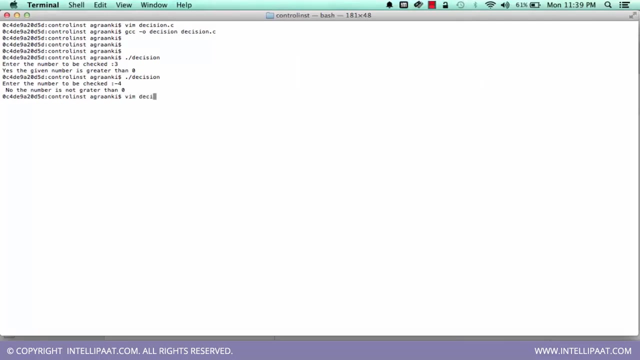 is not true, then structure will check. if condition 2 is correct, if condition 2 is also not correct, then statement. then the else statement will be printed. okay, so let's write some code for this. let me take one example: you, okay, let's write a code, write a program to check if number is greater than 0. 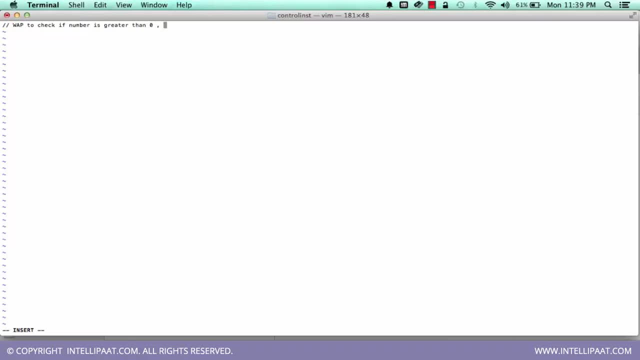 number is divisible by 2. okay, so we are checking two things here, so let me include stdioh hash. include: return 0. int a. I have declared one variable printf. enter the number to be checked. scanf: %d and %a. ok, now we'll be adding the nested if-else condition if a is greater than. 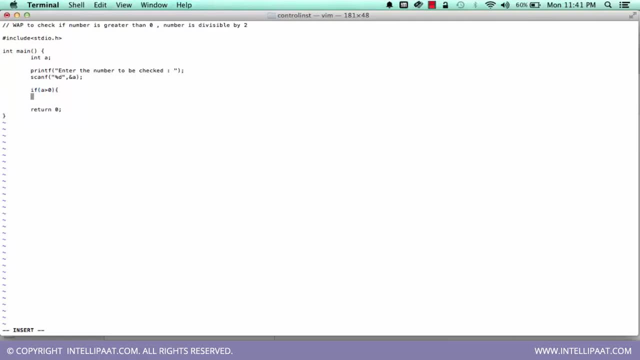 0, then check. yes, if it is greater than 0, then we'll be printing out: yes, it is greater than 0. yes, if if so, this will check if a percentage 2 is equal to 0. if it is true, yes, yeah, Knits divisible by two. else printer a is neither greater than zero. 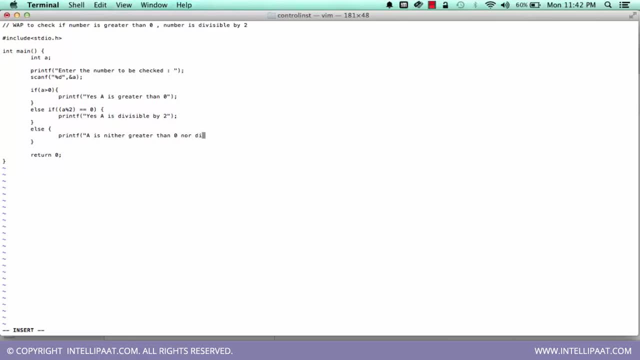 nor divisible by two. okay, we give one more printf so that our output is clearly visible in the screen. okay, let me compile it. yes, the program is compiled quickly. okay, enter the number to be checked. I'll say four. it says yes, the number is greater than zero. I'll run it again. I'll give. 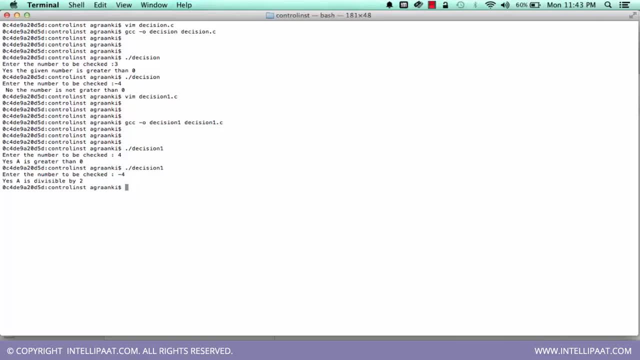 minus four, so it says yes, number is divisible by two. so I'll run it again. I say yes minus five, so it gives me a is neither greater than zero nor divisible by two. so this program checks if a number is greater than zero or a number is. 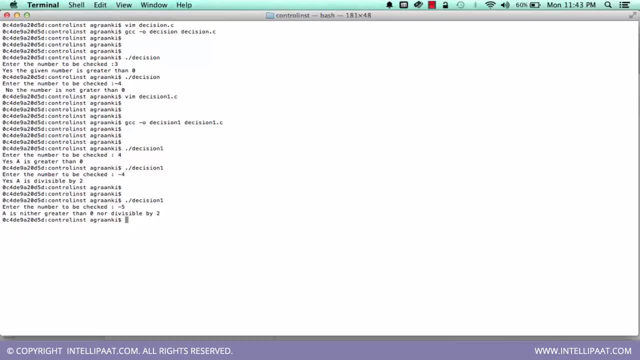 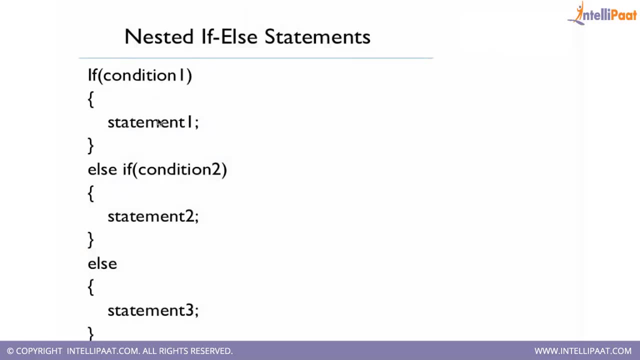 divisible by two. if not, then print that your number does not fall into the given criteria. okay, so here is one more example of nested if and else, where we have two numbers: M equal to 40 and equal to 20. if M is greater than n, then it's printing: yes, M. 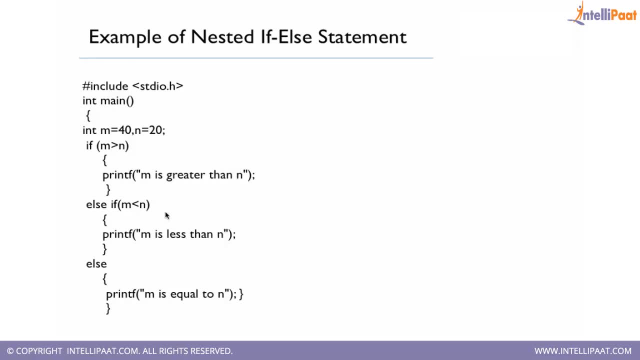 is greater than n. if it is less than n, then it is printing: yes, M is less than n, else if these two conditions are not fulfilling, then it says that M is equal to one. so this is also very simple. so that's it for today's lecture. I hope you. 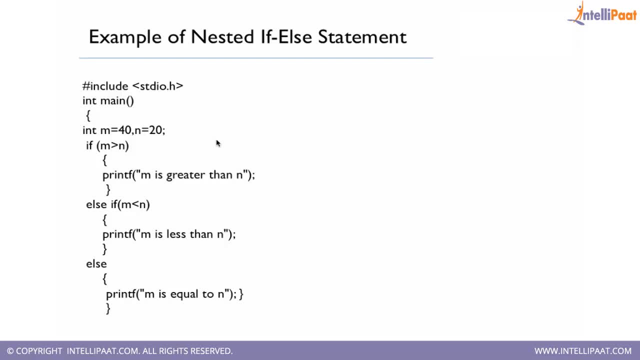 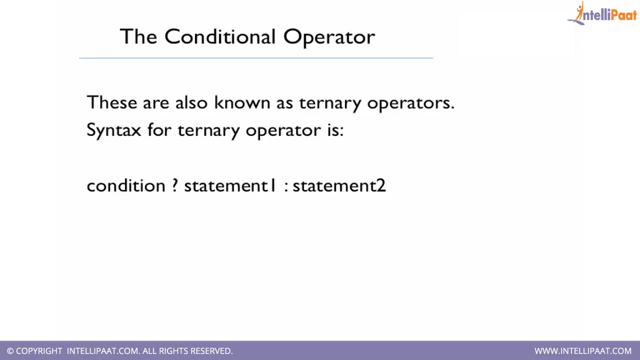 learned something from this video. if you liked it, please subscribe to my channel. simple example: I like you to try it out at your place so that you can get more understanding on the nested, if else statement: okay, the conditional operator- so conditional operator also- is also known as the ternary operator, the 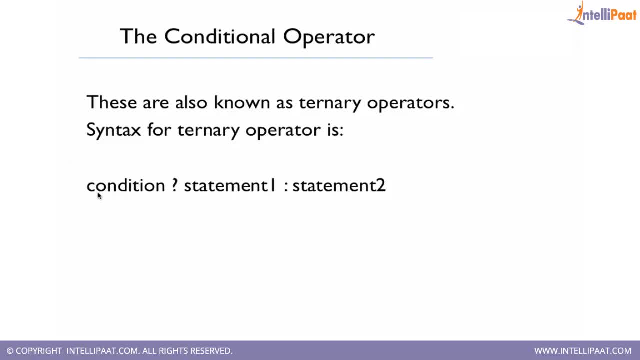 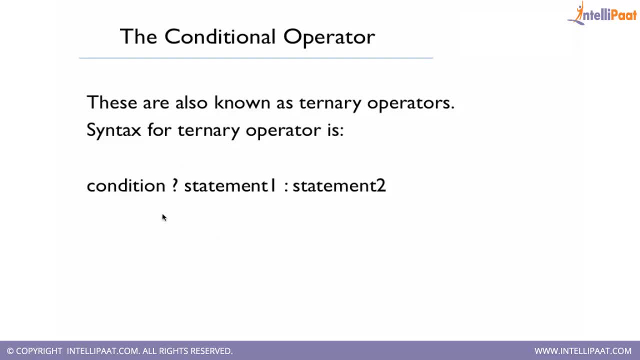 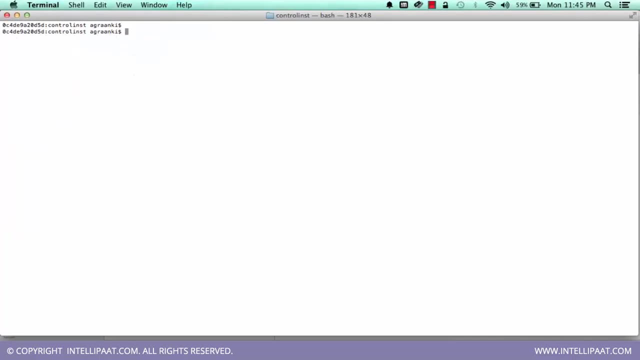 are divided, are separated by some delimiters. so question mark and colon are the delimiters here in this case. okay, so let's write some code for this example. ok, example of secondary operator. so example of a ternary operator. okay, hash include stdi, dot h. main method. let me return 0. now let me declare one variable. 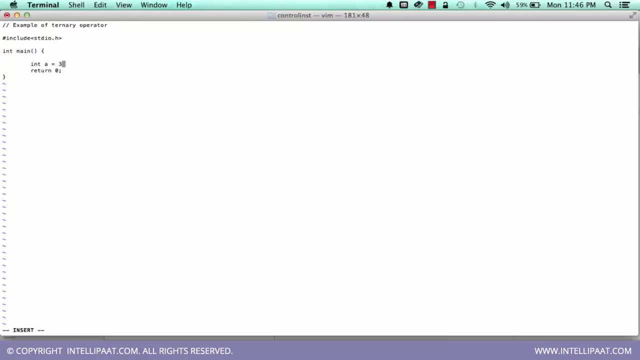 and a equal to say 3. here we'll be checking if the number is divisible by 2. scanf: %d- %a. let's have some ternary condition. okay, if a %2 equal to equal to 0, then printf. let me give the number: %d is divisible by 2. 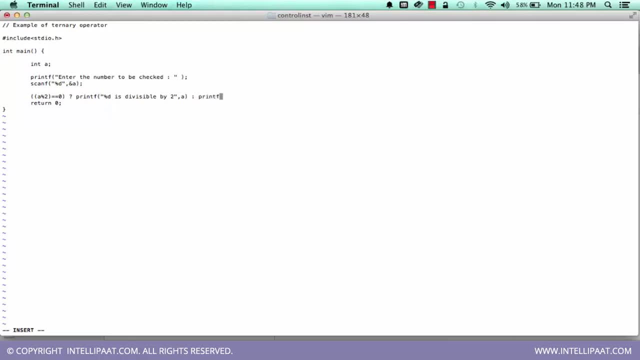 else printf %d is not divisible to a. okay, let me give one printf. this will give me more. this will segregate output. okay, let me save it and compile it. pcc-o. ternary c. compilation is successful. let me run it. okay, enter number to be checked. 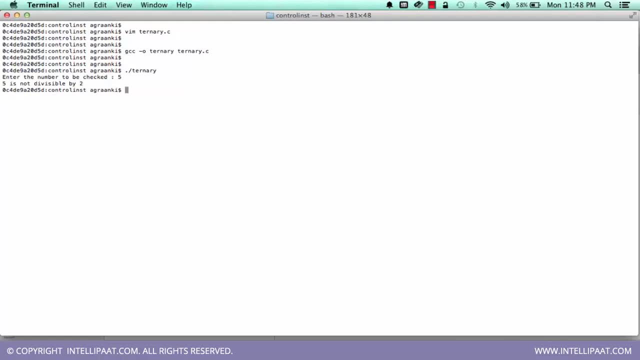 i say 5, so 5 is not divisible by 2. let me run it again. I will give 4. we say 4 is divisible by 2. so this is how we use the ternary operator. so basic syntax is the condition, then statement: in case the condition is true. 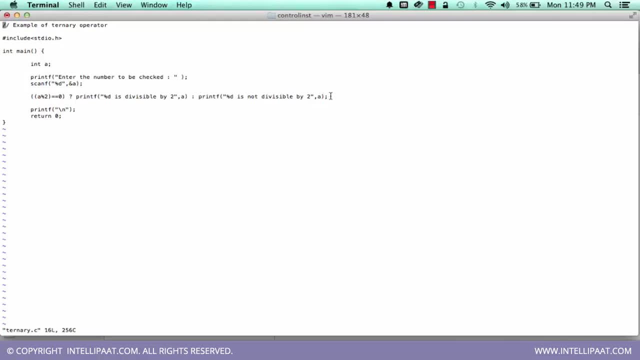 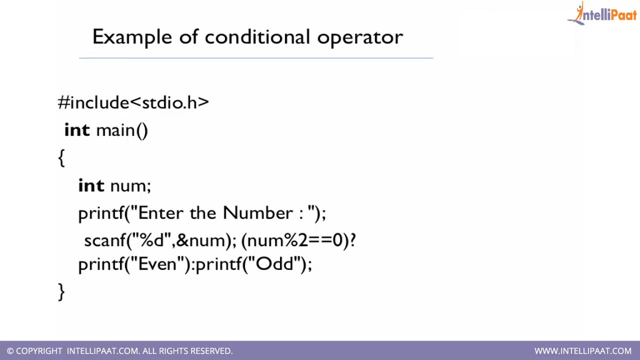 then the statement, in case the condition is false. so this is if statement and this else is treatment. okay. so this example- here I am, I have used the same example- that we have this written the code for, so loop. now let's begin with loop control structure. so what are loop control structure? loop control structure. 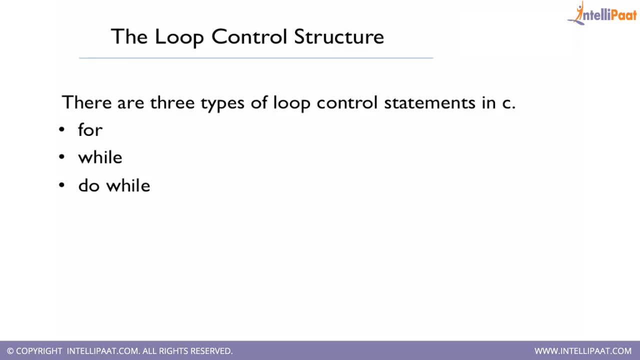 are nothing but structure that facilitates the operation that we want to repeat. it repeat for certain times. C supports three type of loop control structure. one is for loop, one is while loop and one is do I loop. so is it just a basic flow chart of how your loop structure will look like? 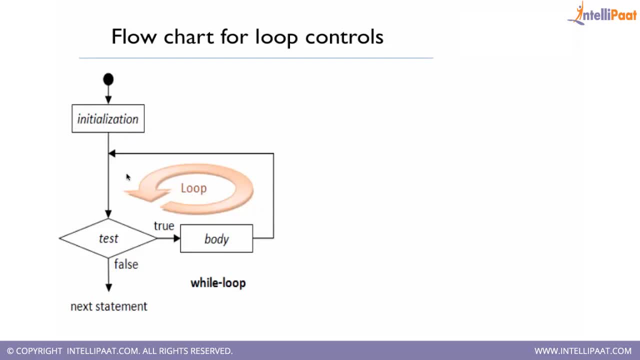 there would be one initialization okay, and a condition that needs to be tested. if the condition is true, the loop will be continued. if the condition is false, the loop will be ended. for example, if you want to print the number from one to ten, I'll be initializing some variable. say: suppose int i equal to zero. 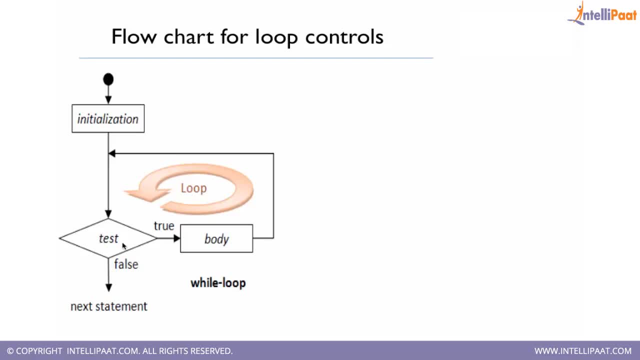 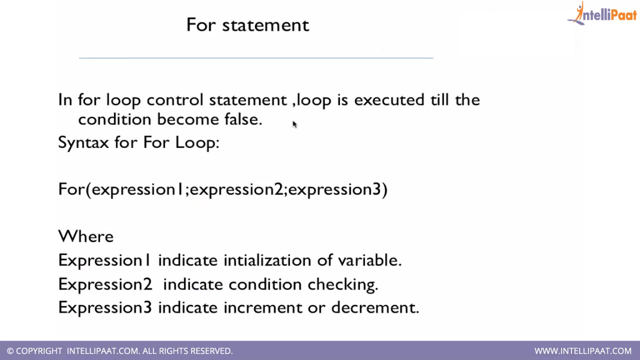 and check if i is less than ten. if the condition is true, I will be doing some. can we doing some calculation? or I will be doing some other stuff? the condition true, I will be following it to false, false. so let's see what. what is the syntax of? 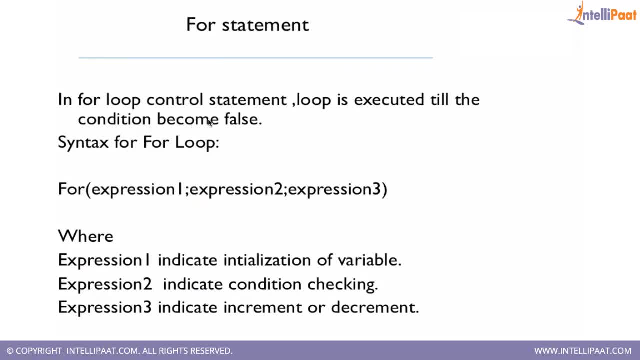 false statement. in for loop control structure, park loop control structure, food. so let's see for. for statement is true, but this problem will be a love statement, so let's see what how much well becomes from our one. haven't found only conditions being while inbundle control. if we have Cave any else, alabama, okay. 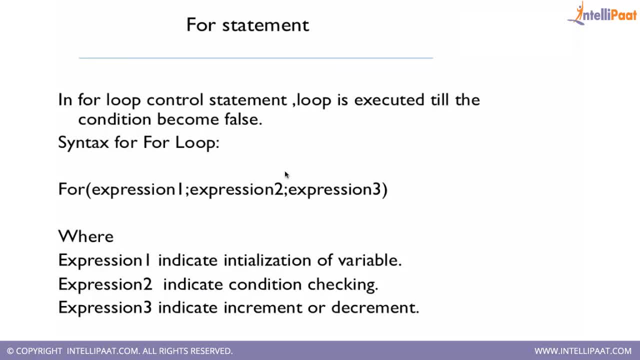 loop is executed till the condition becomes false. so this is the basic syntax of for loop. we have expression 1, expression 2 and expression 3, so expression 1 indicates initialization of variable, expression 2 indicates condition checking and expression 3 indicates the increment or decrement of. 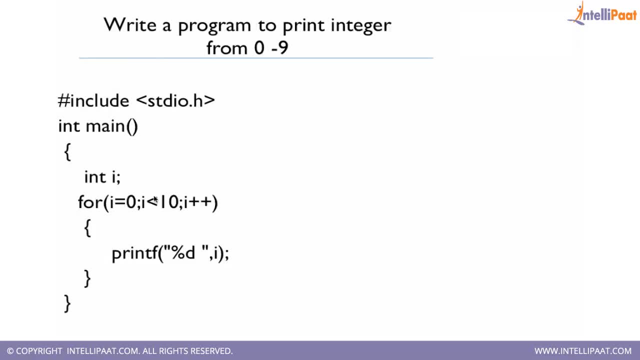 the variable. so here is a example. in this example we are printing a number from 0 to 9. hash include std error dot h. int main. int I. I am declaring I now. I am initializing I to 0. I am checking I is less than 10 and incrementing I by 1. 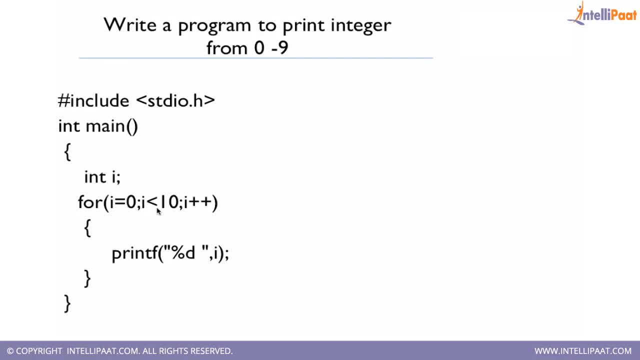 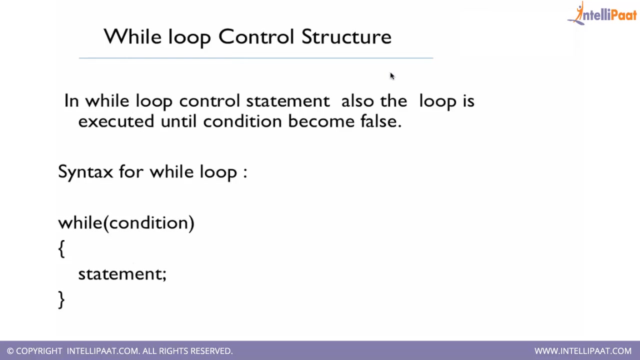 and here, if this condition is true, I'll be getting inside the loop and I'll be printing the value of I. so this code will result in printing a number from 0 to 9. okay, so for while loop in while loop control structure the statement also. 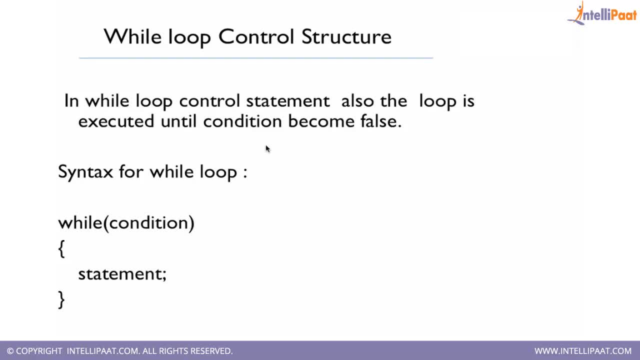 the loop is executed until the condition becomes false. so here's the syntax of while loop. so here syntax of while loop is while condition and statement. so in while loop we need to make sure how we are checking the condition and how we are exiting out of the loop if we don't do the condition check and don't make. 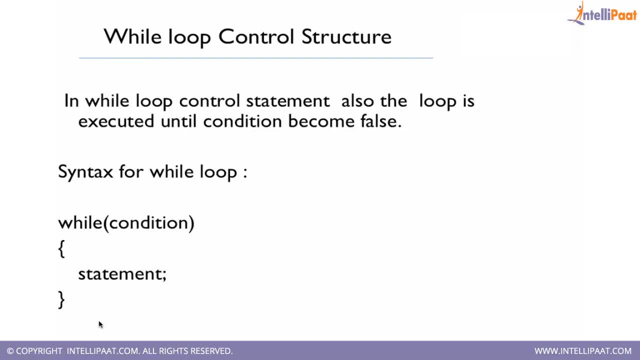 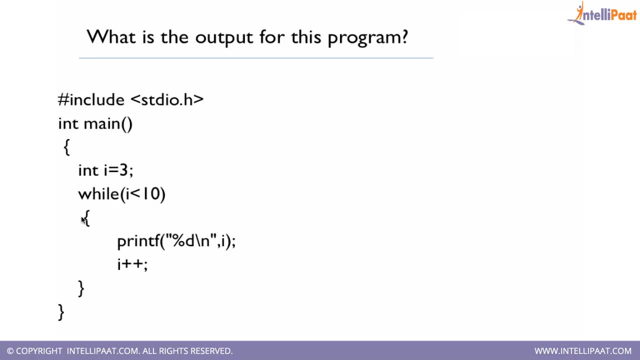 and if you don't make sure that we are coming out of the loop, we will be stuck up and into an infinite loop, and this is really bad. so this is a sample program for writing the while loop. here I am in initializing a variable, I equal to 3, I'm saying, while I is less than 10, I'm. 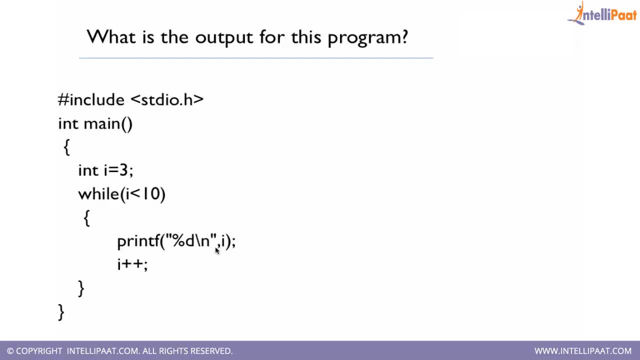 printing on the number and incrementing it. so this, this is very important and this, this is also important. so what? what will happen? the loop will continue till my value of I will become greater than or equal to 10. if I remove this condition, then I have initialized: I is 3, I will always be 3. 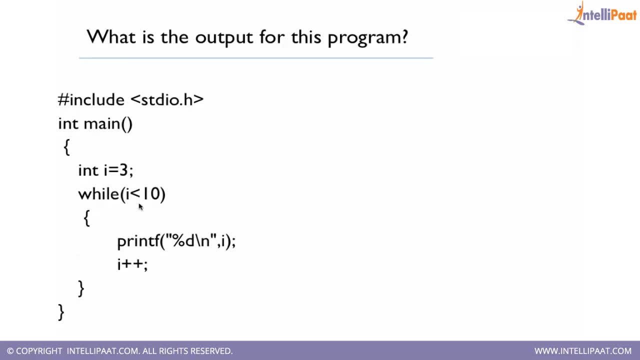 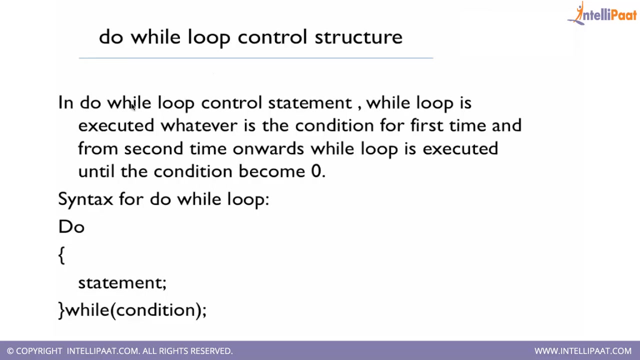 and the loop will continue endlessly. so to make sure that the loop will exit properly, we should have some logic in place so that at some point of time this condition should become false and will be exiting out of the loop. so this is a do while control structure. in do while control structure, the while loop is executed, whatever. 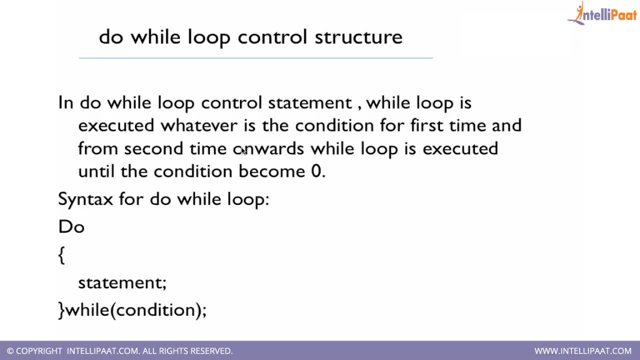 is the condition for the first time, and from second time onwards the while loop is executed and the condition becomes false or zero. the syntax for do while loop is do, and then we are doing one statement and while condition. so in do while loop the statement will get executed. 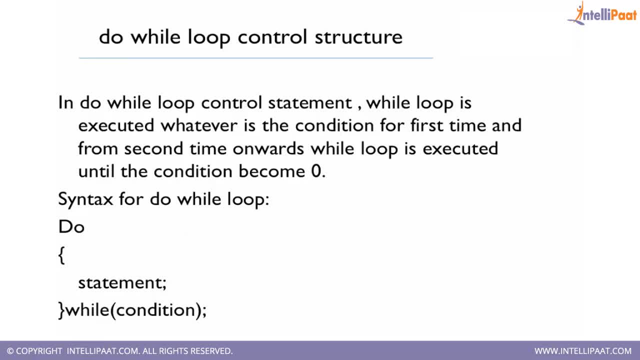 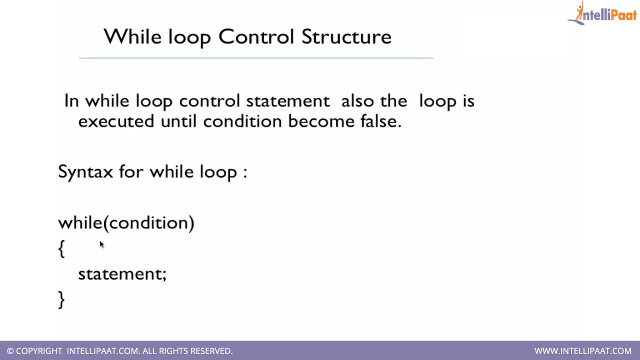 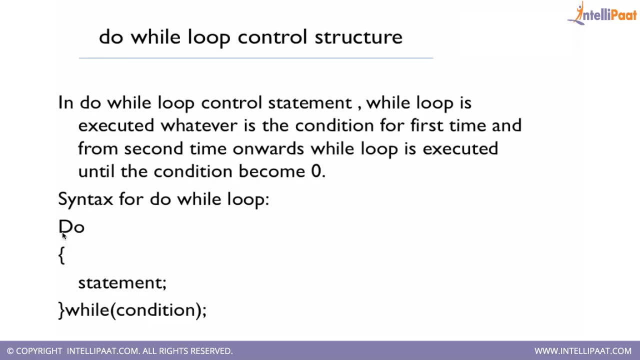 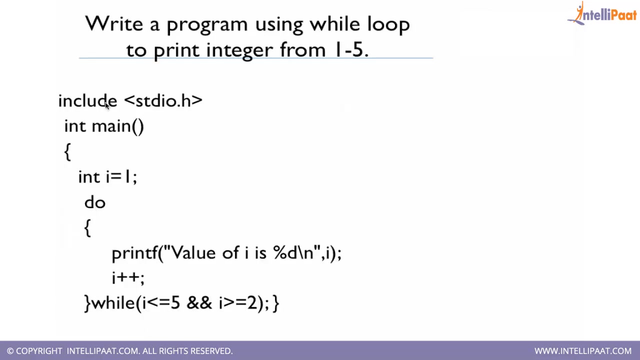 at least once. so first the statement is executed, then the condition will be checked in while loop. first the condition is checked, then the statement is executed. so it depends upon our logic whether we want to use a do while loop or whether we want to use a while loop. so here is an example of using a do while loop. again, i am. 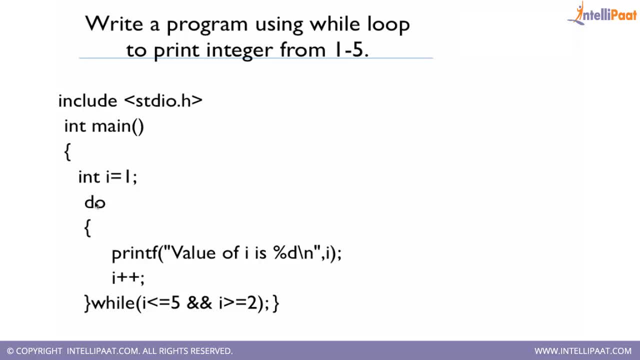 initiate taking one integer, i, equal to one. i am using a do while loop: do printf value of i is, say, percentage d, and then incrementing i, while i is less than equal to five and i is greater than equal to two. so, for the first time, what will happen? the i is one. this 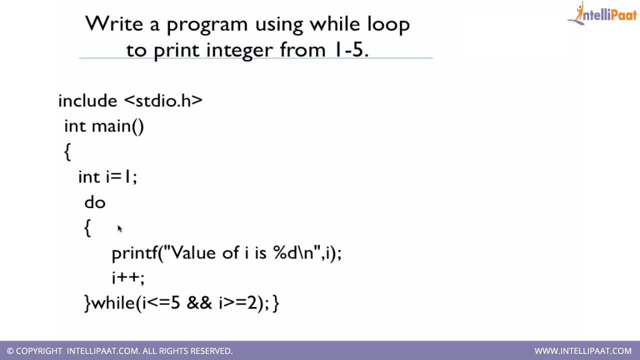 condition will be executed and then i will be incremented in the. at now, at this point of the time, the, this condition will be checked whether the i is less than equal to five or i is greater than equal to two. so when, when this part of code is executed, i becomes two and this condition will 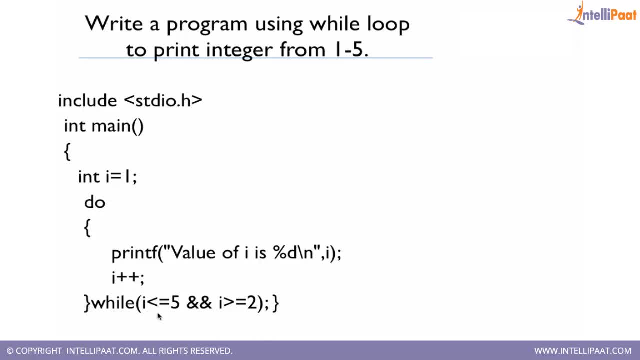 become true. so this loop will be continued, and this will be continued until and unless here i becomes greater than five. so what i'll be printing? i'll be printing one, two, three, four, five. so let's do some, uh, let's write some examples or some code for all the loop structures. 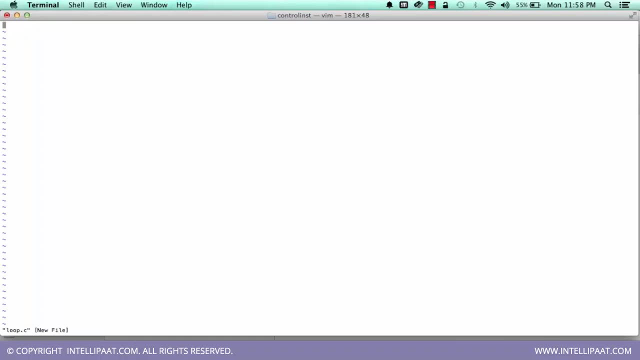 okay, so let me include a studio dot as so: 0. okay, I first. I'm using a for loop, for loop, for I equal to 0, I less than 10, I plus plus. okay, I am printing. I printing, set HD in for loop. let me print hi. okay, so this will print the value. now let's let me have a while. 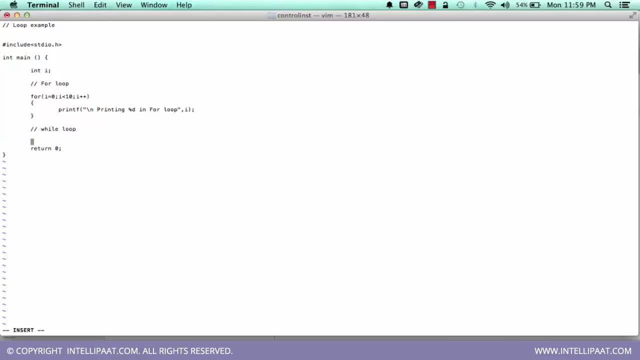 loop. okay, so I'm initializing I with 0 again, and so while I is less than 10 printf, slash n printing percentage in while loop I, and I mean incrementing I. this is very important. now let's use do while loop I equal to 1, 2 printing, sorry, and F. 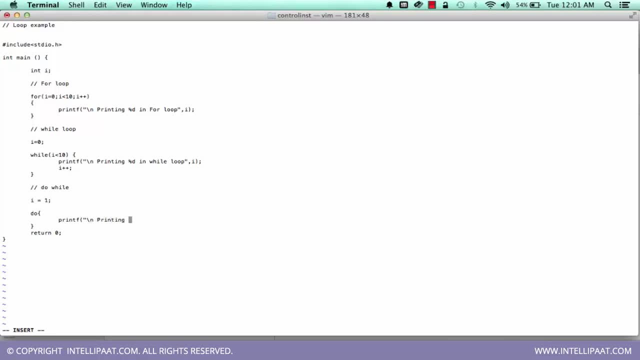 slash n printing percentage D in loop I and I plus plus, while conditions: while I is less than equal to 5 and I is greater than equal to 2. okay then let me give a printf here, the slash n, so that outputs is clearly visible. okay, let me compile this code: ECC minus O, loop dot C. 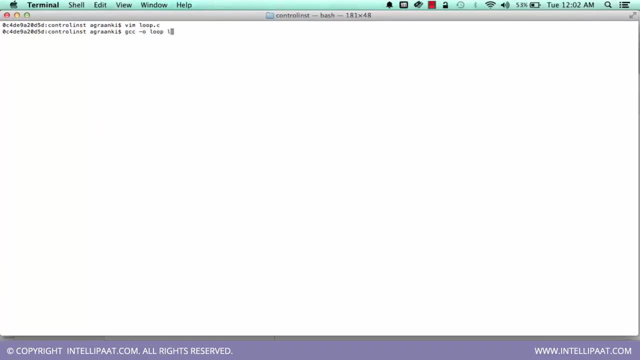 minus O loop dot C. yes, code is compiled successfully. let me run this code. so here we are. we got this output. first we have printed 0 to 9 using for loop. then we have printed 0 to 9 using while loop. then we have printed 1 to 5 using do while loop. okay, I have combined the examples of for loop- while loop. 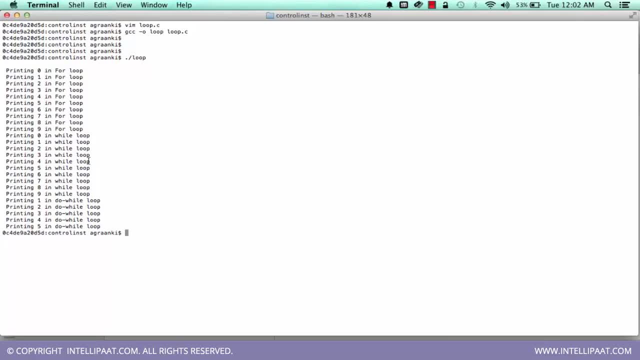 and do while loop in one program. so just to make sure how to use these things. so it depends upon your program logic, on how you want to make sure how the conditions are executed. only the iterations will remain the same, like how you want to use iteration when you want. 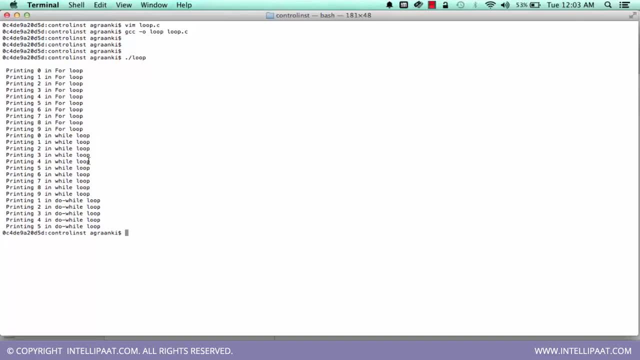 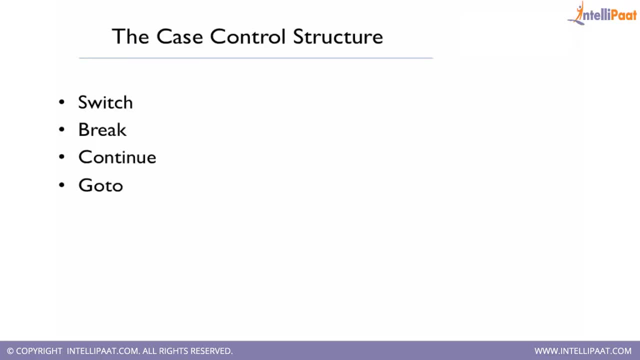 to make when you want to check the condition and incrementing the variables, decrementing the variables and so on. so case control structure. case control structure is a special type of control structure where we can check one condition for or one event for a multiple actions. for example, we, if we. 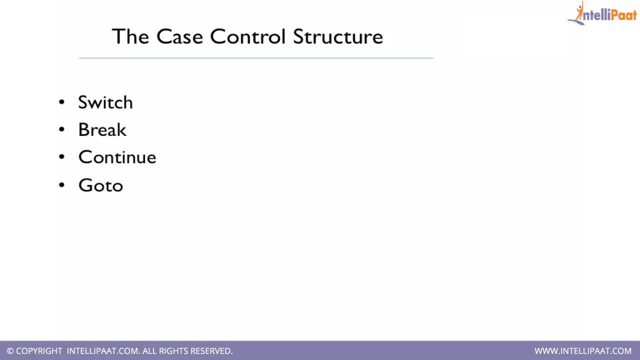 want to check if number is number is greater than zero or number is divisible by two. so we can easily write a very simple if case case control structure to solve. this case control structure has following keywords: switch, break, continue and go to. we will be covering this right. 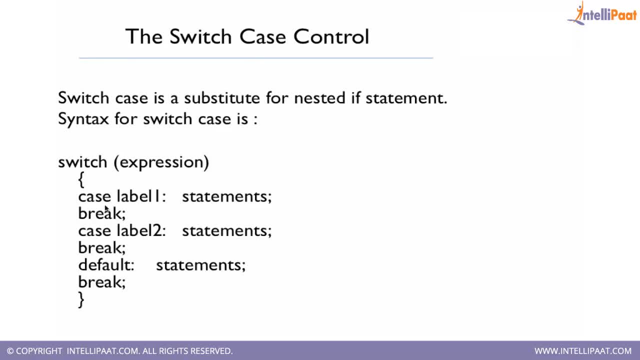 now. so how we use switch, switch and case. switch switch case is substitute, substitute for nested if statement. so earlier if you, if you remember, we have written a program for nested if a statement where we have checked if a number is greater than 0 and or a number is divisible by 2, we will be writing a same program using switch case. 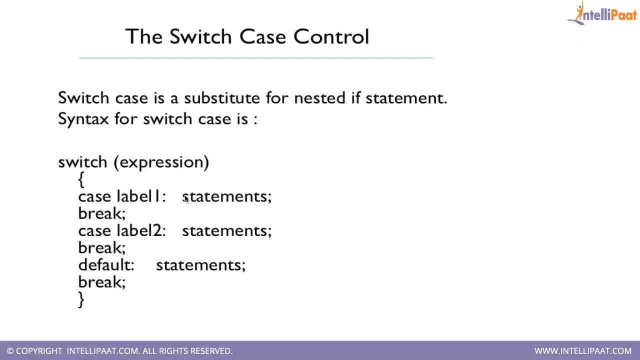 statement. the syntax of switch case statement is like this: it will have a switch then expression, then it will be having a corresponding case statement, then break case statement, then break default statement and the break. so how this is executed, it will check the condition if the condition my matches with any of the 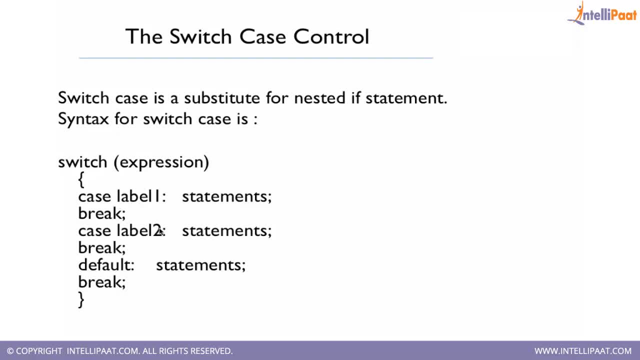 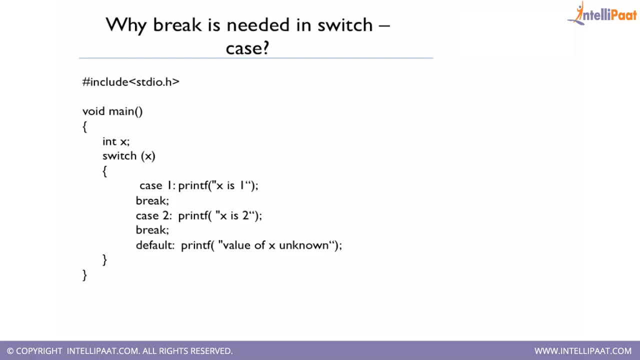 label, it will execute the statement corresponding to that label. if the any of the case is not matched, it will execute the default statement. why break is needed? because if you don't give break here, suppose let's consider this program, for example. we have a program widen like this: wide match. 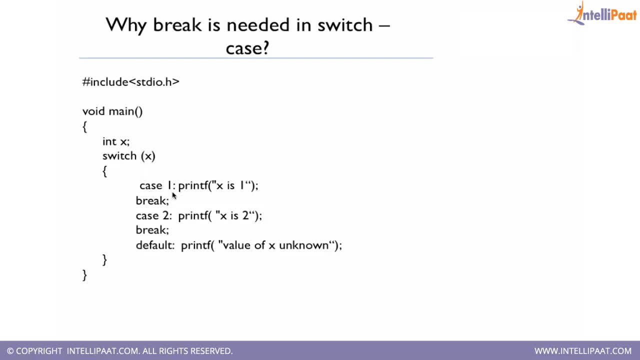 main in tax, which it's is one case to and and default. for example, if x is a one I will be checking for, really of x, it falls into case one and it brings case 1 if and it breaks here. so if I don't give a break here, it will, it will. 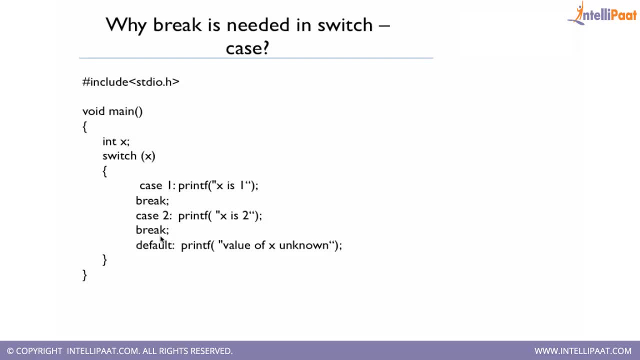 continue the executing the case statement until it founds a break. so suppose, if this break is not here, this break is not present and I give X equal to 1, I will be printing: X is 1, X is 2 and now, until and unless it identifies a break- and now this is a wrong- my value of X is 1 and 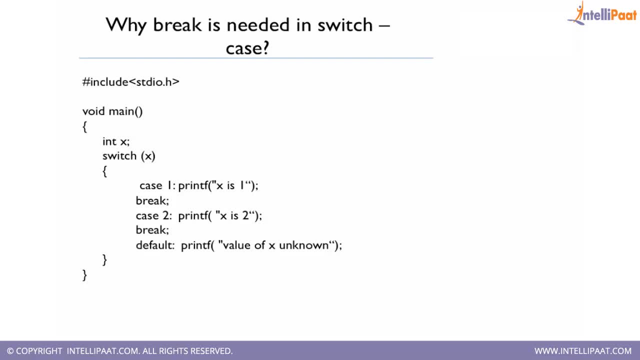 I am printing: my X is 1, X is 2, so we have to be very careful to use break where we want to use break. what is our logic? and we should be exiting the cases case statement as and when is required. so this slide explains why we require. 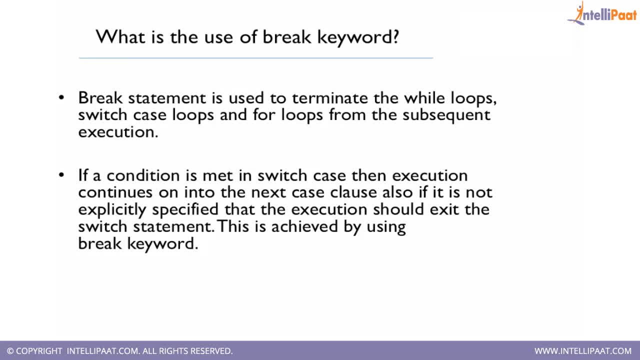 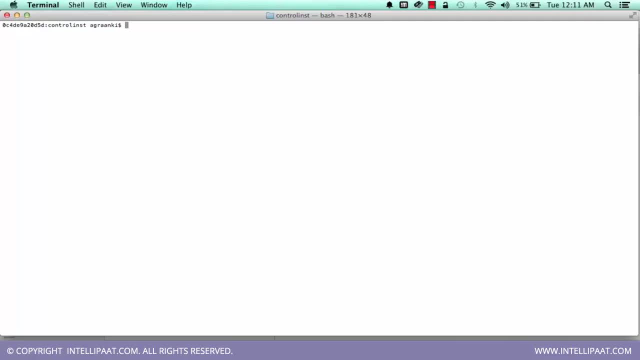 the break keyword. so let's write some code to understand how case is written. Search case control structure works program to understand switch case structure. I'll be including a still data here. Now I have to print break dot. edge hash mean zero. okay, let me have some integer, say integer x. let me get an. get it input from user. 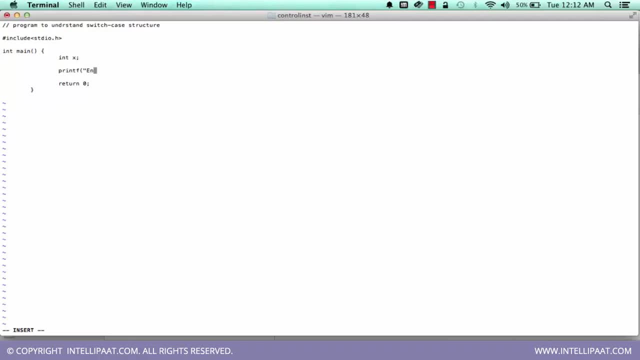 value of X. scanf percentage D ampersand x: okay. scanf percentage D ampersand x: Okay. scanf percentage D ampersand x: okay. okay, let's use switch X, case one. printf you: X is equal to well, let's check if a number is divisible by 2. so X percentage: 2: okay. 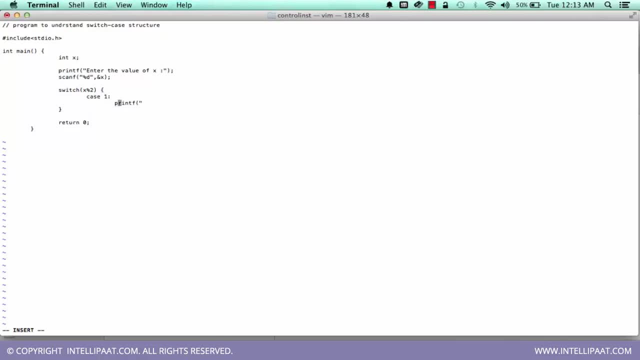 is one: X is not divisible by 2. break case 2: case 0. printf: X is divisible by 2. break. let's have a default says in path. it says I don't know the output. okay, let's give a printf here, let's save it and compile it. 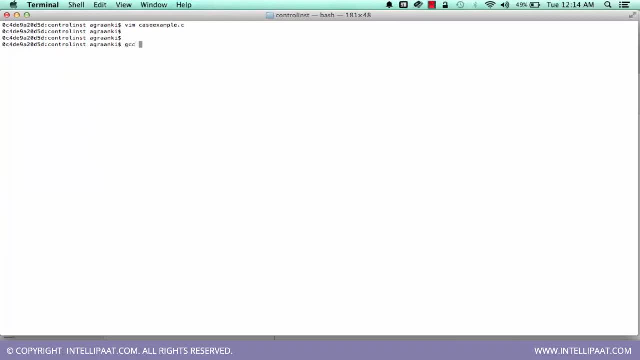 so compilation is successful. let's run it. enter the value of x. i'm saying five x is not divisible by two. let's run it again. i am giving: say two x is divisible by two. let's run it again. let me give some negative value: x is divisible by two. so this is how switch case behaves. let me modify the. 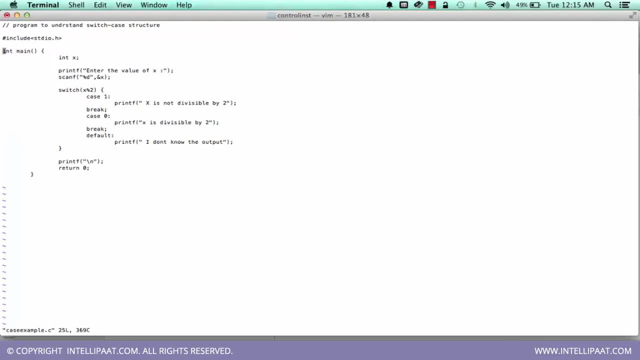 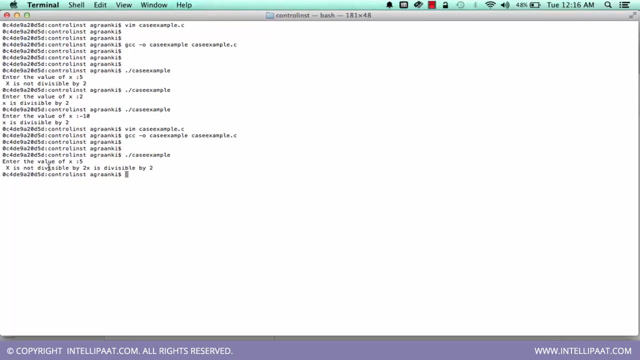 program. okay, so what if i remove this break statement? let me comment it out. okay, so let's compile the code again. let's run it again, enter the value of x and say five, so it gives me two output: x is not divisible by x is not divisible by two and x is divisible by two. so if i remove the break, 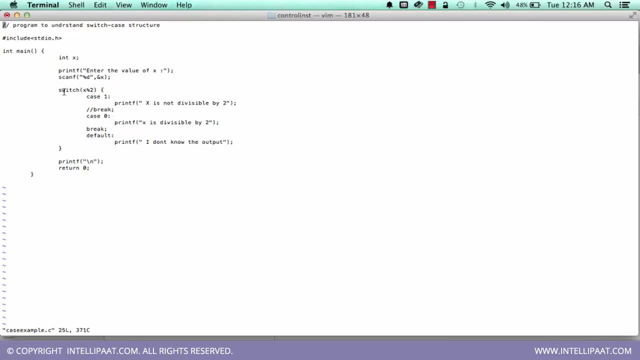 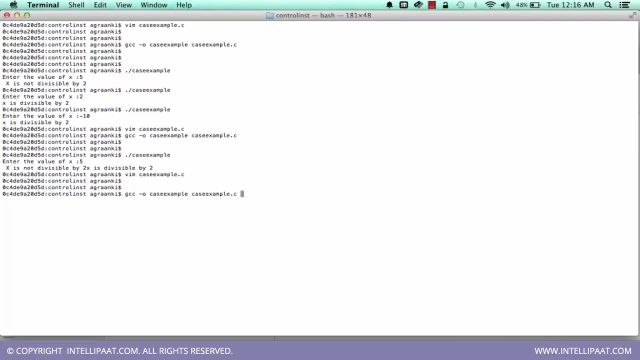 it will execute this condition. since I have given 5 X person, 5 percentage, 2 is 1. it executed this condition and it didn't find a break, so it also executed this condition. it finds break here and terminated at this point of time. let me remove the comments and let me comment out this break. let's compile it again. 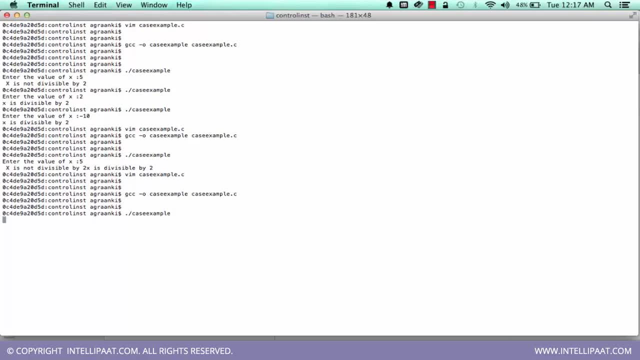 then it again enter the value of X. let me say 6, it says X is divisible by 2 and it says I don't know the output. let me run it again. if I say 5, it says X is divisible by 2. let's revisit our. 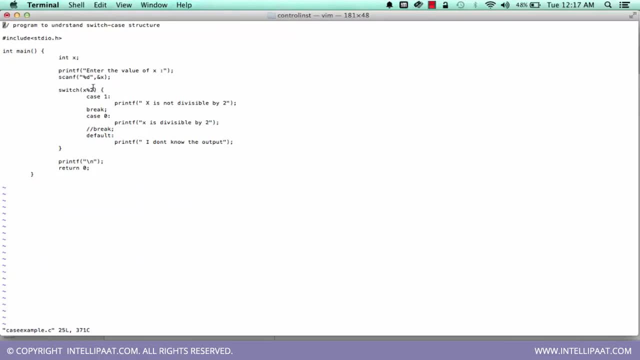 code. so in this case, if I give 6, 6 percentage 2 is 0, it comes here. let's say: X is divisible by 2 and there is no break. so it will continue till the switch statements ends or it finds any break. if I give 5, then 5 percentage 2 is 1. it came here this: 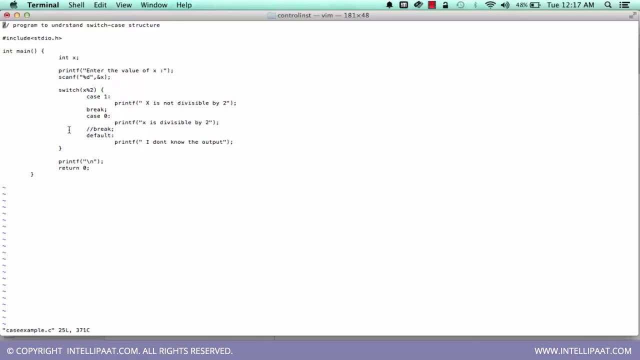 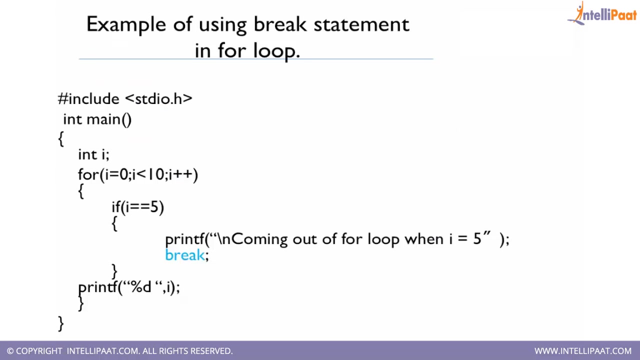 statement is executed and break. so that's how switch case works. so be very careful to put breaks wherever is required, otherwise you are not going to get the correct output. so example of using break statement in for loop: so break statement can be used in loops also, in suppose, if you are want to exit the loop prematurely. 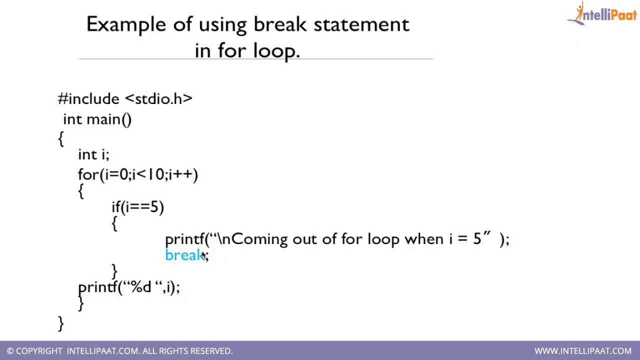 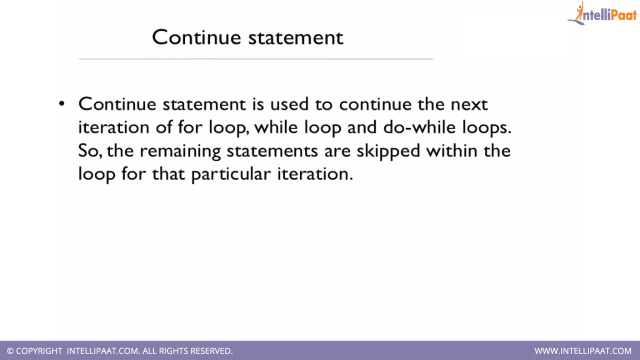 from some condition. you can put break and you can put break, and you can put break and loop will not be continued. we will be exiting out of the loop and the statement after the loop will be executed. so this is how break in loop work: continue statement. continue statement means: 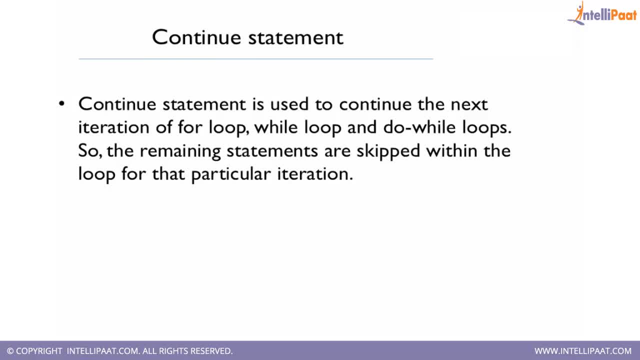 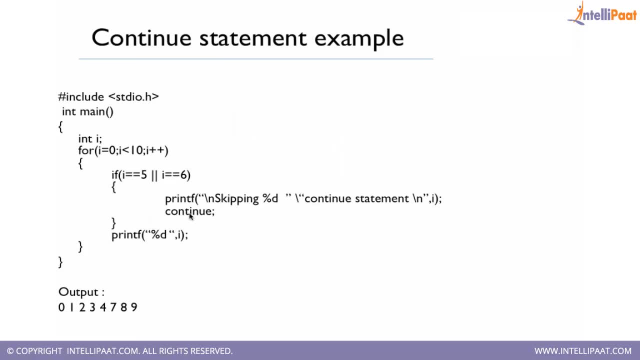 continue statement will continue the loop, like it will check if some certain condition is true or false. if we put a continue keyword inside a loop and if the loop hits the continuous condition, then what it will do is it will not execute the statement after continue, but it will go to. 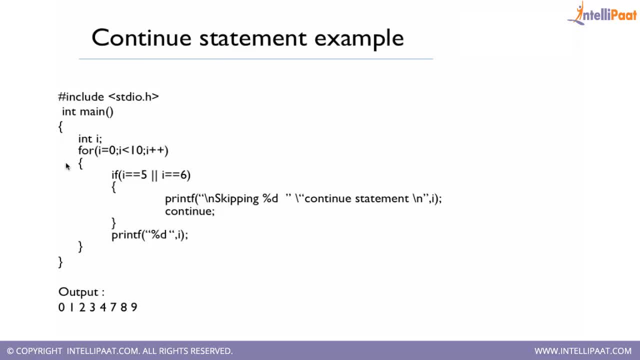 the next iteration of the loop. loop will not be executed, but it will go to the next iteration of the loop. so you can see, for example, in this case we are printing a number from 0 to 9. so if this condition is matched- say I equal to if I is 5 or 6- we will be skipping the. 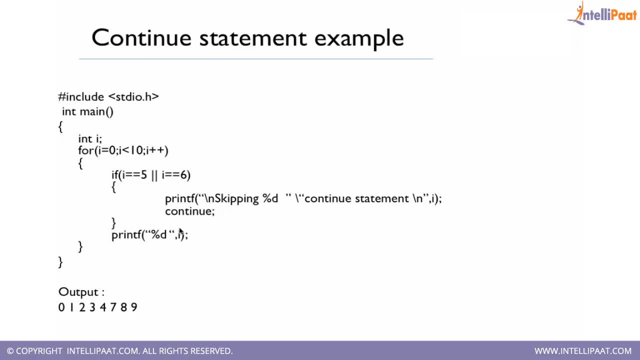 execution of statements where we don't want to execute. in case I is equal to 5 and 6, so we have kept continue. so in this place my output will be 0, 1, 2, 3, 4, 5 and 6 will be skipped. 7, 8, 9. so because this printf is not shown in the output, 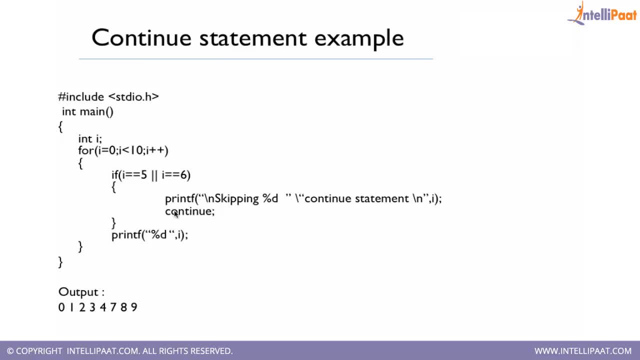 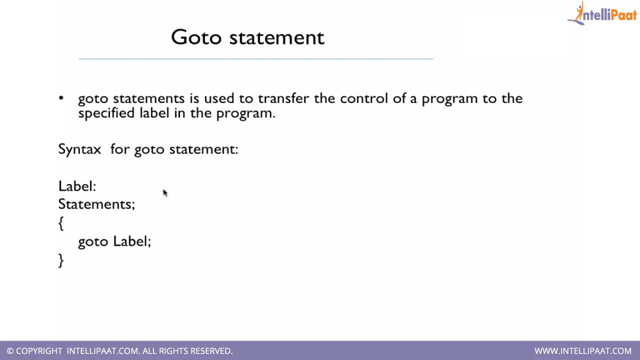 but yes, this printf will be coming into output. but just to make and just to explain how continue works and this is a a. this is how the continue works. if we comment out this print statement, this is the output that I will be getting. so goto statement, goto control structure is: 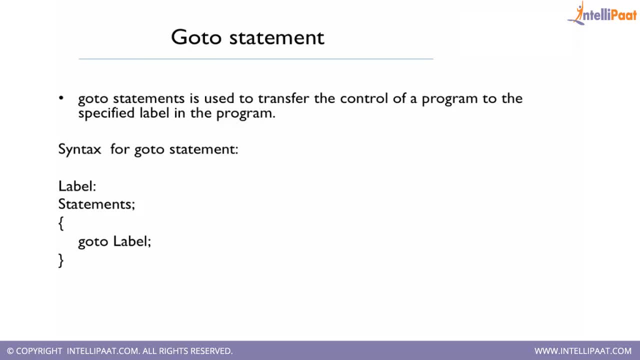 used for to transfer the control of a program to a specified level of a program. so it is kind of looping. but C has provided goto but it. it is advisable not to use goto control structures because you never know when your program will going to misbehave. so it's always advisable to use either. 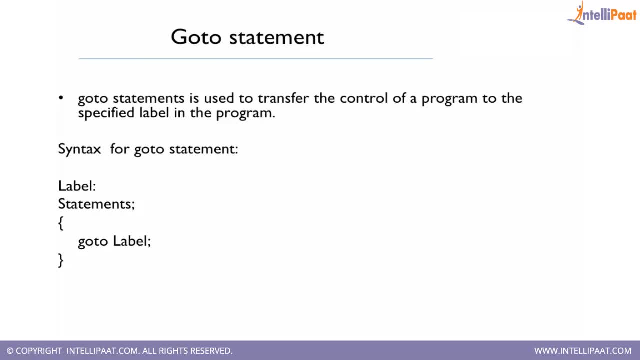 standard loops like for loop, while loop, do while or some if a statement switch case but be and I'll. I'll advise not to use goto statement because that can lead to a very buggy code, since C support this, so I will be covering goto in this lecture. so this is a syntax of goto statement. we. 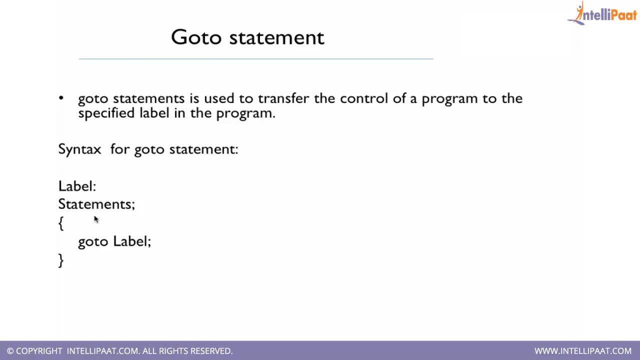 will be having statements goto label. so when the statement is executed, when I hit the goto, I'll be directly going to place where label is there. so this is kind of looping from here. I'll jump directly here, then I'll be executing this. I'll be jumping here. 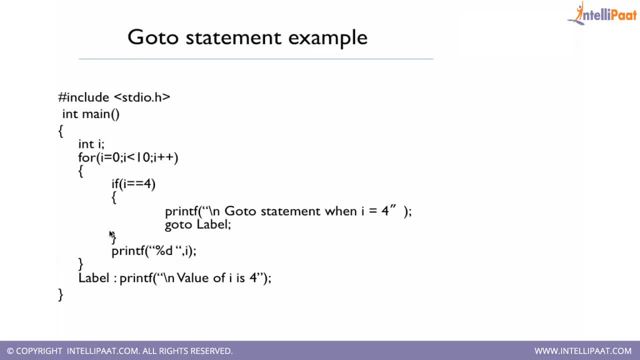 again, this is the example of how goto is used. so this is a code: int main and I equal to- sorry, I have declared I for I equal to 0. I is less than 10, I plus plus. if I equal to equal to 4, printf goto statement. when I is 4, say goto label, and in this case the loop will be exited. so if I is not equal to 4, I'll be printing the value. in case I is 4, I'll be exiting out of the loop. so this is how goto works. so what we? 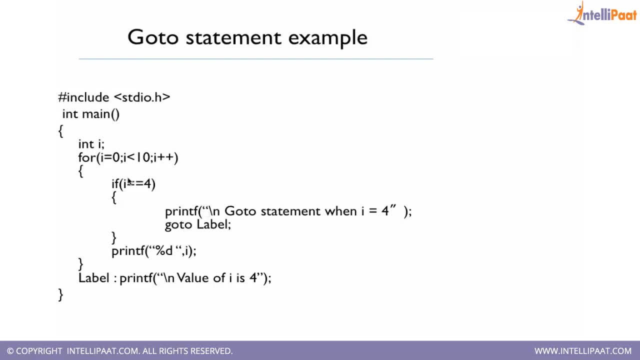 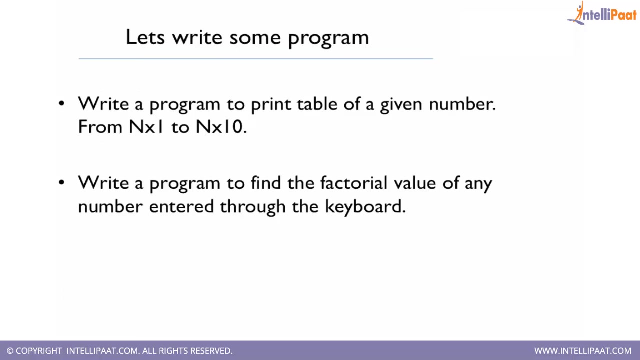 be the output of this program. the output will be 0, 1, 2, 3 and when 4 is executed. next time that is printed is go to statement. when I equal to 4 and value of I is 4. this is the output. so let's do some more coding, let's write some more. 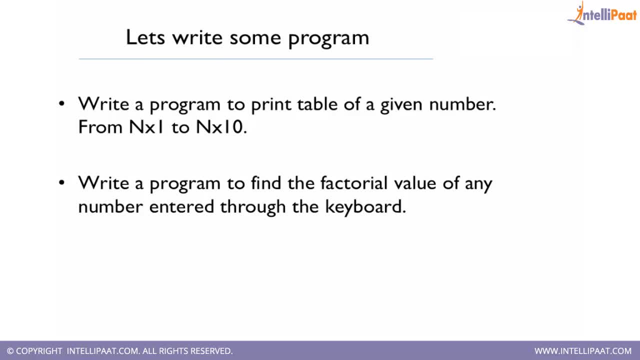 program. write a program to print table of a given number. for example, if I am given a number, say 9, I will have to print a table like 9 into 1, equal to 9, I need to equal to 18, so on till 9 into 10. so let's write the code for this. 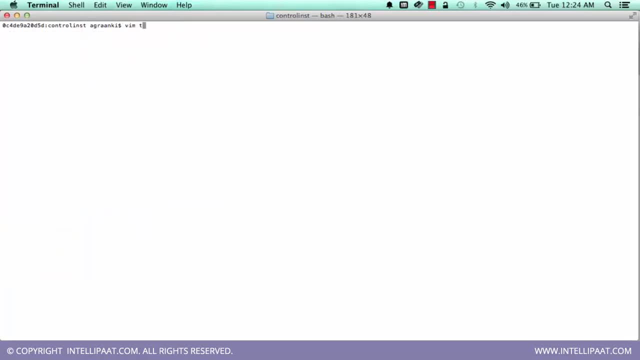 okay, let me include stdi. you dot, edge mean and I am declaring some variable: I and n. let's get an input from user, enter the number, scan it: percentage d and percentage n. now for loop equal to 1 I less than equal to 10 I plus plus. I'm printing and def. 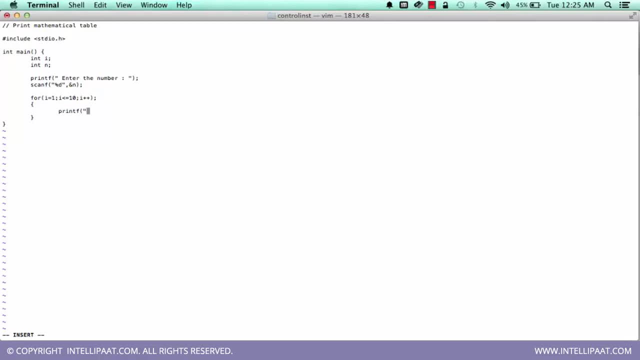 I percentage d into percentage d, equal to percentage d. okay, so let me and slash and next time, and knows how? have we come today i case we call the deploy never name? in order to show you how I code here, and let me just apply a public name. 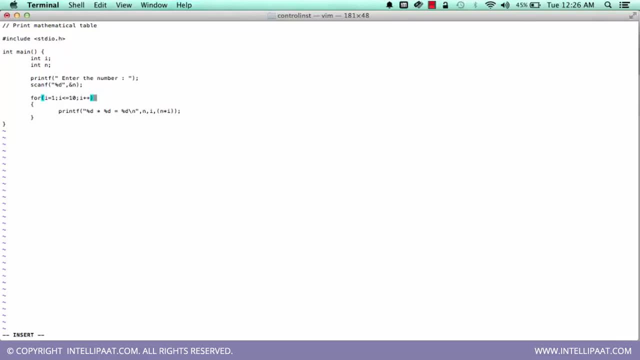 and those commands are not needed. i got my public key, kind of webradул, so that's enough for me. it's gonna be fine. okay, program is successfully compiled. enter the number 9. so this is how I am printing: 9 into 1, equal to 9,, 9 into 2, equal to 18,, 9 into 3, equal to 27,. 9 equal to 4. 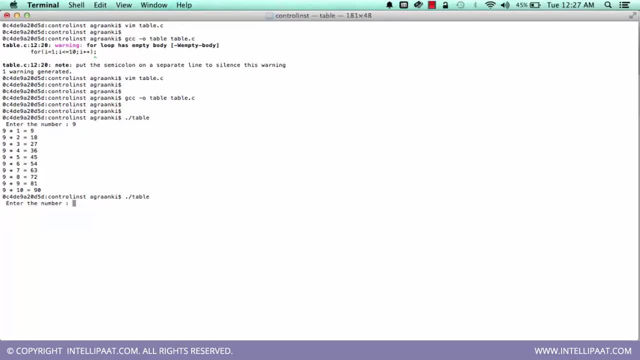 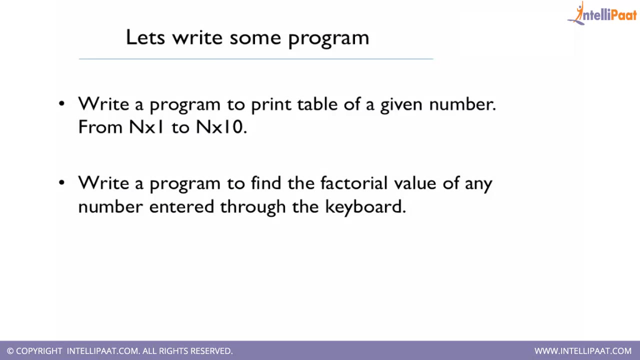 36. let me run it again. let me give, say, 16, so I will be getting a table of 16. let's do one more code at a program to find the factorial of any number entered through the keyboard. so how we calculate a factorial: the factorial is calculated. 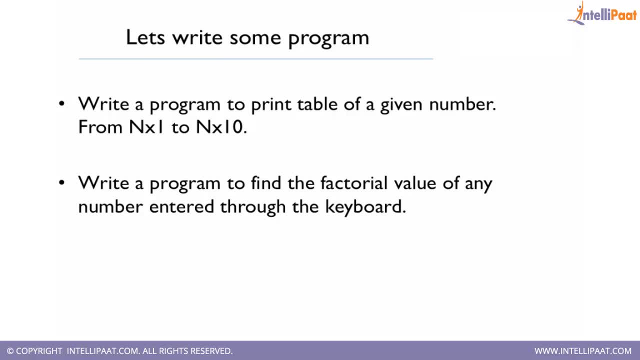 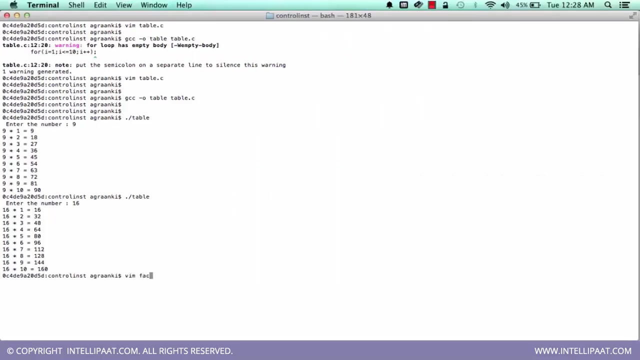 suppose you have number n, so factorial is calculated as n into n minus 1, into n minus 2 up till n 1. so here also we need to do the loop, create a program for this. so we are printing factorial of a given number in this program. 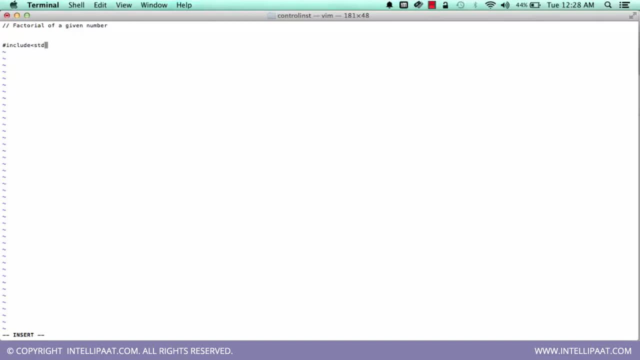 hash include STD, IO, dot H and then return zero. and then let's get it from user and if and and percentage, D and percentage. and okay, now let's take a while loop here using one more variable. I equal to one, and I'll be using one more. 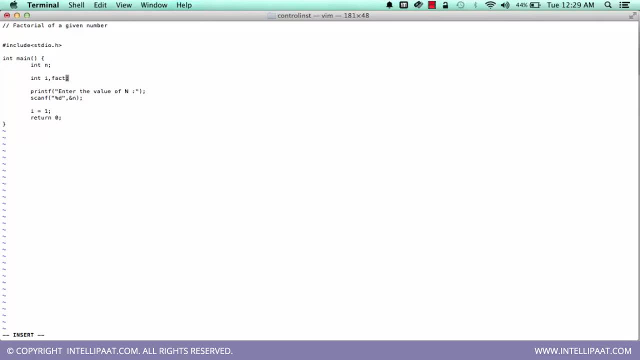 variable say factorial so and factorial also equal to one. okay, so I will be writing a loop. while I is less than or equal to n factorial, equal to factorial into I, let me implement I. okay, Now let me print the output: factorial of percentage d is percentage d so factorial. 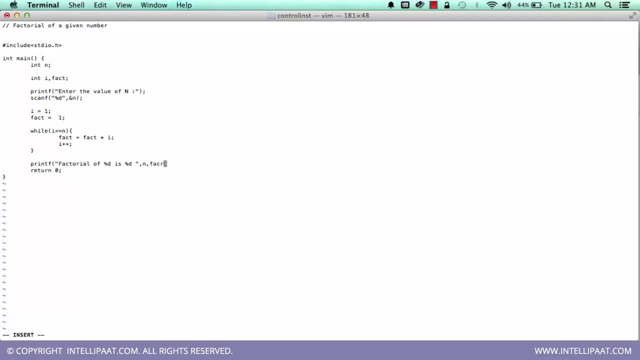 of n is FACT. Let me give one slash in here. So this is how we can calculate a factorial. Let me save and compile GCC minus O. Okay, program got compiled successfully. Enter the value of n, let me say 4.. So factorial: 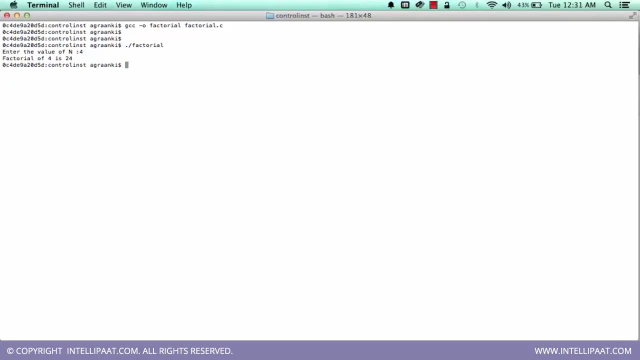 of 4 is 24.. So this is correct. Let me run it again. Let me give, say, 6.. So it is giving me factorial of 6 is 120.. So this is how factorial is calculated. Let me save. 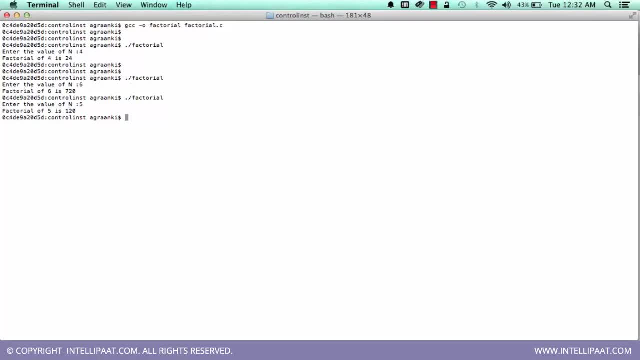 Let me run it again. Let me give 5. It will give me 120.. So this is how factorial is calculated. We will be here in this program. We are going from 1 to n and multiplying the factorial every time with i, incrementing i. 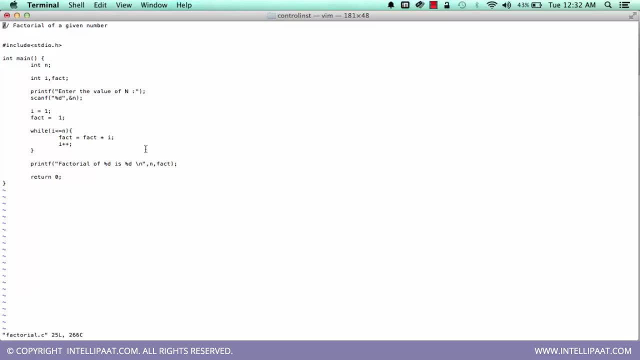 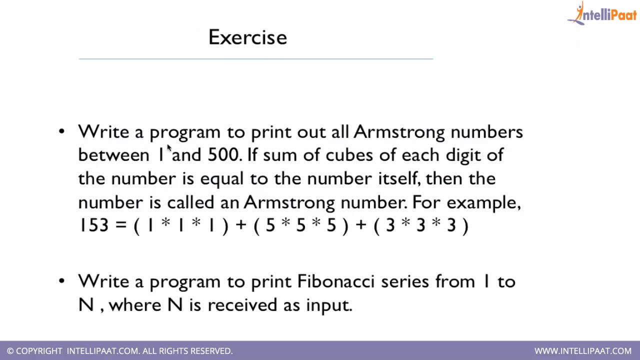 So, and at the end we are going to get this: Okay, We are printing the output. Okay, So now I will be giving you this, these two exercises. you can try it out at your place. First problem is write a program to print all Armstrong numbers between 1 and 500. 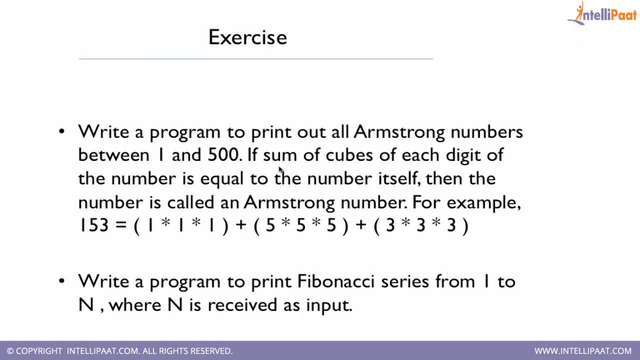 So what is an Armstrong number? If a sum of cubes of each digit of number is equal to the number, then the number is equal to 0.. number is called Armstrong number. for example, 153 equal to 1 into 1, into 1 plus 5 into 5 and 5 plus. 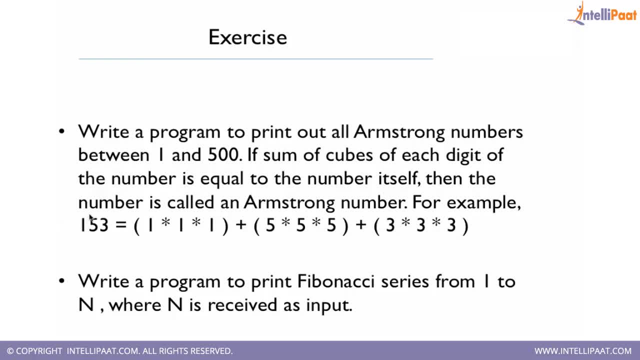 3 into 3 into 3, so the cube of every digit, sum of cube of every digit, is equal to the same number. then it is called an Armstrong number. so you need to write a code. this will also. you can solve it using one of the loop and using one of the arithmetic operator. basically, you have to use 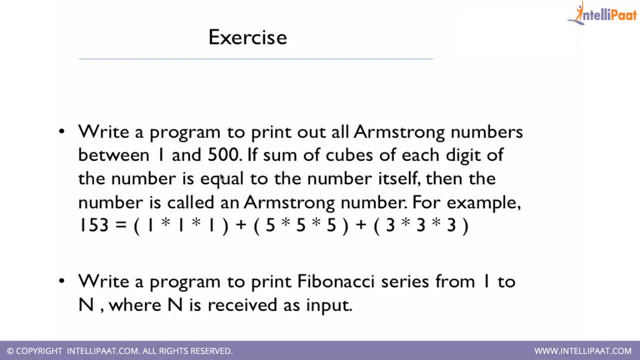 a modulus operator and you can solve this problem very easily. one more program is write a program to print Fibonacci series from 1 to n, where n is received as an input. so what is a Fibonacci series? Fibonacci series is: starts with 0, 1 and then